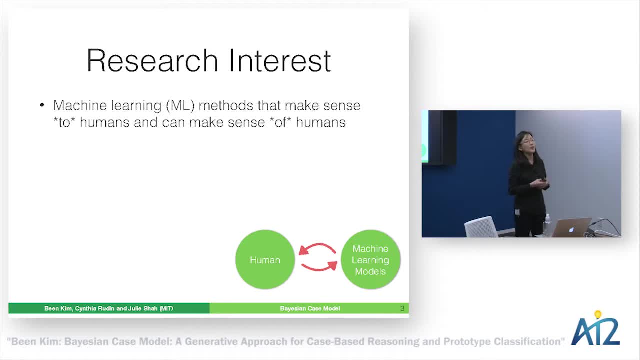 So my research interest is to make machine learning models that make sense to humans and can make sense of humans. And this comes from a really simple goal of my research and my work in general: that I wanted to do something useful. I want people. 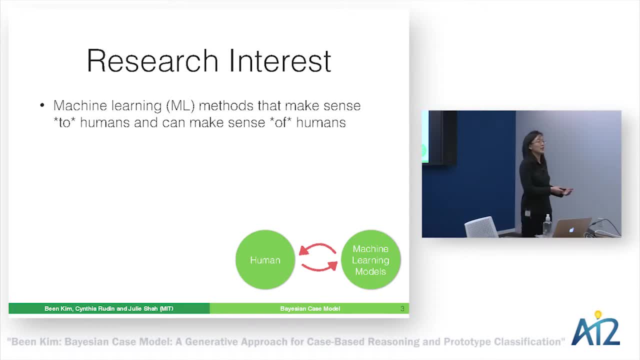 This amazing tool called machine learning. I want people to use it to solve their own problems, But this is not easy. In particular, I'm interested in having normal people who doesn't really know machine learning being able to use machine learning. This isn't easy, because to be able to convince them to use this potentially good hammer, we need to convince them this is doing something that makes sense. 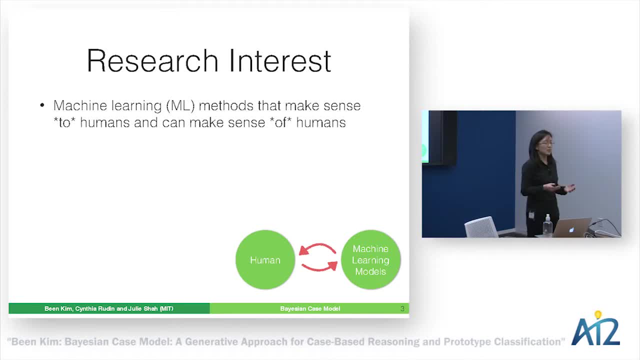 For disaster responders, for example. for these people there's no way they're going to make important decisions- who's going to who you're going to save first- just because computers tell you that that's the best answer. So first way to make this machine learning tool useful is to make transparent systems such that humans can understand. it makes sense to humans. 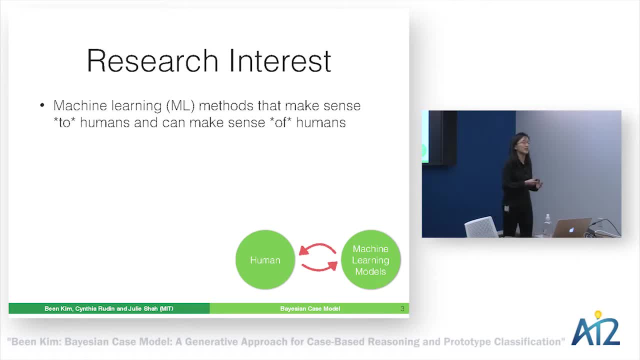 Also, this hammer called machine learning isn't perfect. There are years of accumulated experience of human domain experts, such as disaster responders, that machine learning, machine learning models just don't have. So on the top of that, we need to make sure that machines can make sense of humans so that we can incorporate their feedback back to machine learning systems. 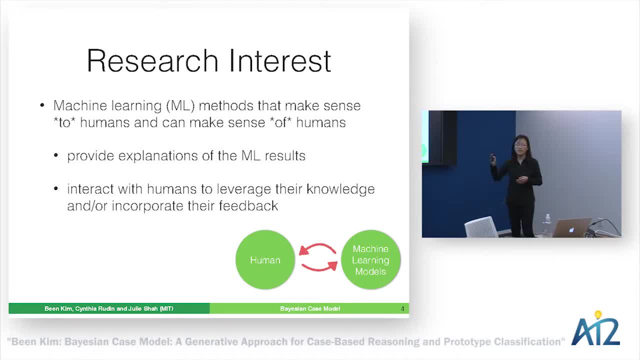 There are lots of different ways to achieve this goal, and here are two things that I've tackled. One is building machine learning models that could provide insights and very intuitive explanation about the machine learning results And, second, making this system that could interact with the humans, so that we can incorporate their feedback back into machine learning systems. 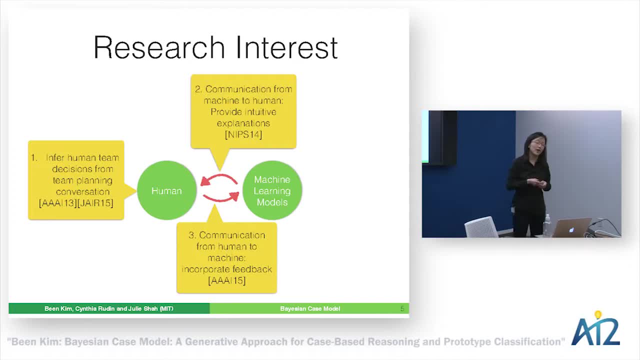 Breaking down my research even farther down. I worked on these three different areas. Today's talk I'm going to mostly talk about number two, which is the communication from machine to humans. How can we provide intuitive explanation from machines to humans? But I want to touch really briefly on 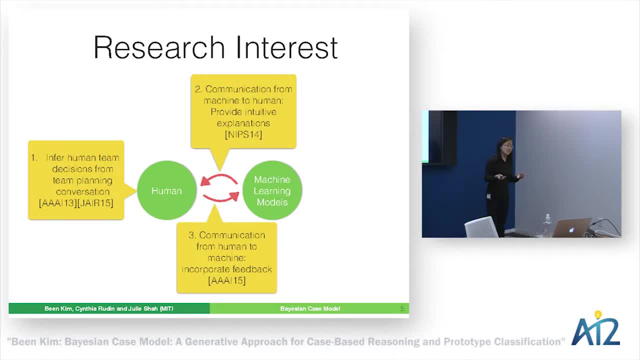 what I did for the number one. This is how we can make sense of humans without machines getting involved. So if humans are discussing, in particular discussing their plans for disaster response, can we infer what they are talking about? And this is to make sure that if machines have suggestions as to better strategies, 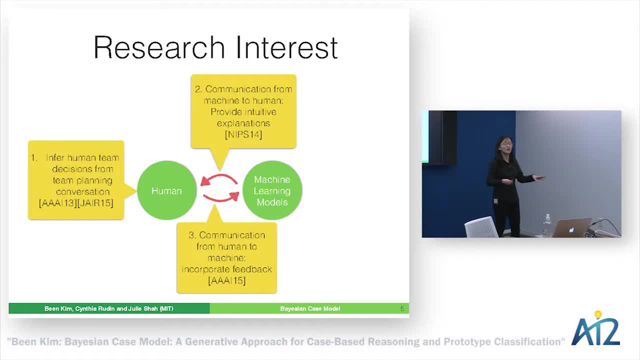 then we need to know what humans are talking about first, so that we know when to make the right suggestions and what kind of suggestions we need to make. So the first part of my PhD work is about given a dialogue, about making plans for disaster response. 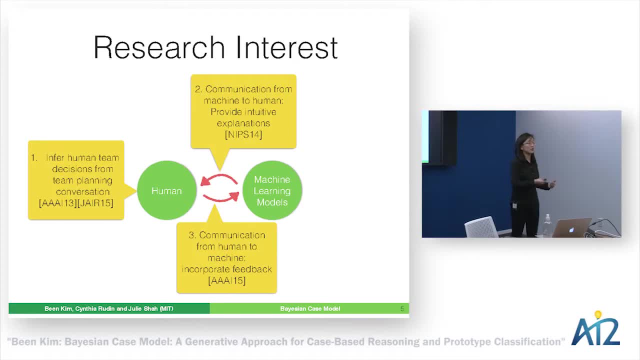 can we infer what humans finally agreed upon. So we show that that's possible. And then the next step was OK. well now how can we intuitively communicate machines' suggestions back to humans in a very intuitive way, And that's the talk that I'm going to give today here. 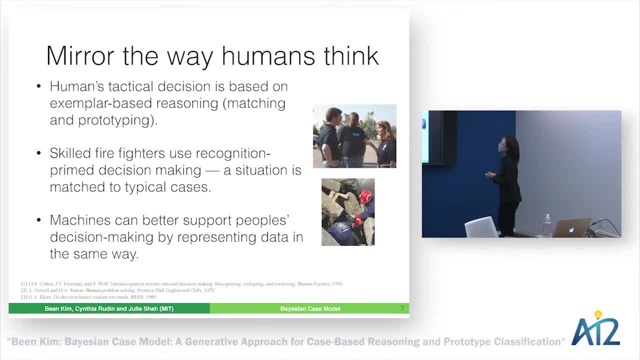 So the first thing to think about when we want to communicate with humans is to think about how humans think. In particular, I'm interested in improving decision makings for domain experts such as disaster responders, When humans are making tactical decisions. there's a lot of rich literature that shows that humans make exemplar-based reasoning. 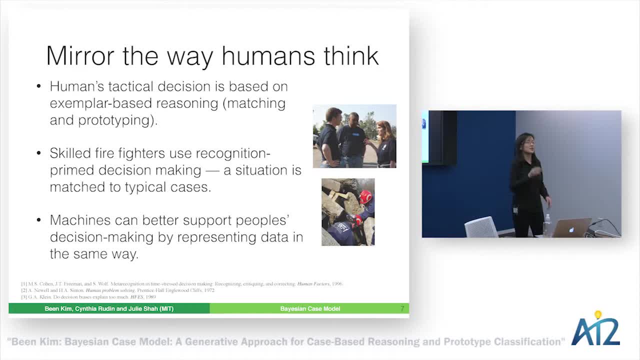 And this is just a fancy word, for humans recognize the new incident, for example, as a type of previous incidents that they have dealt with, and apply the modified solutions to their new incident, And, in particular, a skilled firefighter does exactly this. 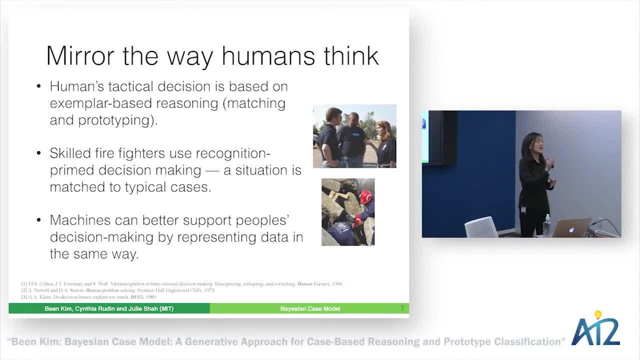 They have a new fire and they identify: oh, I've seen something like this in 1996, let me modify my solution and apply to that. That was successful, let's do it. And so the idea is to for machines that can better support human decisions. 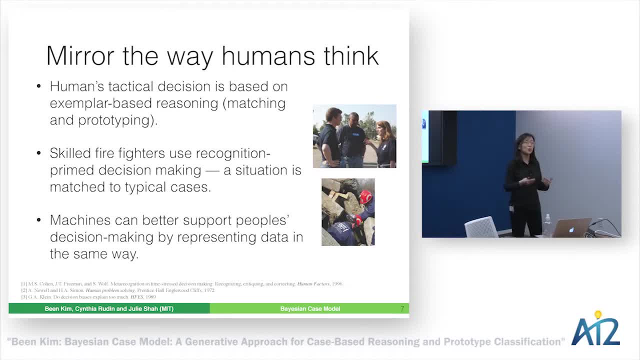 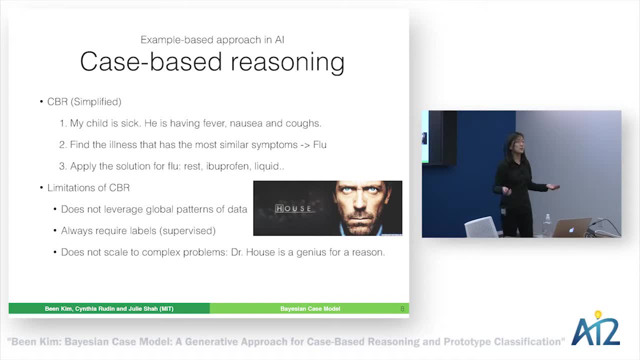 we need to present the information in the form that humans think. So that's where we came about. let's use examples to explain machine learning results to humans. This is not a new idea. this has been very successfully studied. classical AI called case-based reasoning. 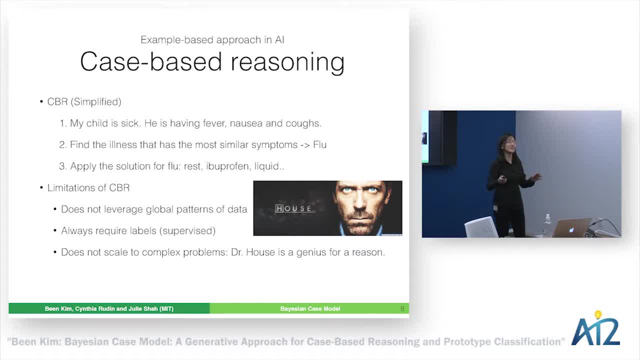 So case-based reasoning is a very fancy name for something quite simple. actually, we do it every day. Let me give you an example of case-based reasoning. Let's say your child is sick, he's having a fever and he's nauseous and having some coughs. These are the observed variables. you're observing these symptoms of your child. Then what you do is find the illness that is closest to the symptoms that you see, in which case here it might be flu. Then you apply the solution for flu to your child. 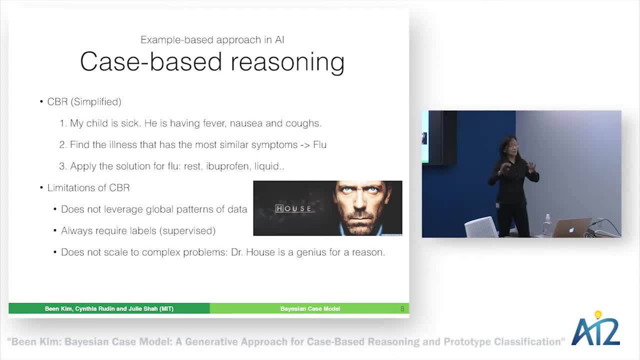 There's routine and feedback loops in the details of case-based reasoning, but this is a basic, simple idea that we actually do on a daily basis. So this powerful idea has achieved a decent success in healthcare and manufacturing and other real domains. But CBR comes with limitations. 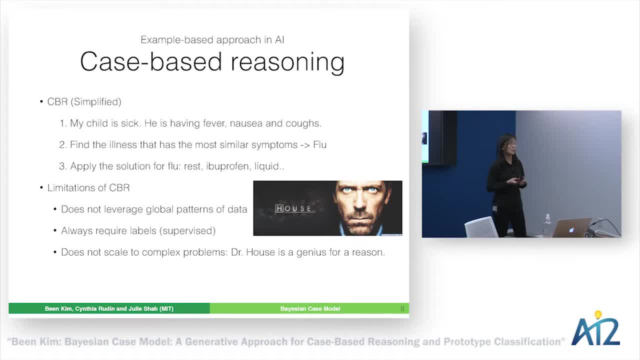 CBR does not leverage global patterns of data So, for example, there is maybe food poisoning in the cafeteria of the school that your child is going to temporarily. maybe last week something happened, so a lot of kids are sick with that and you know it. 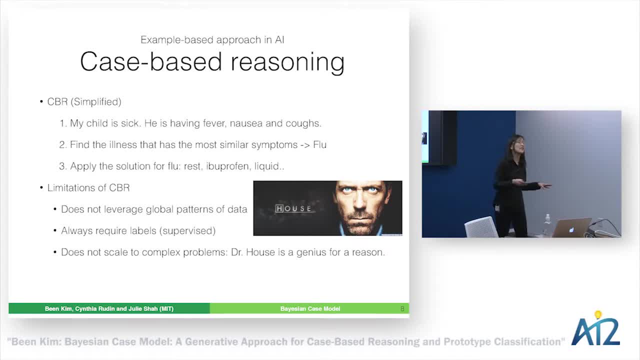 But CBR doesn't know how to leverage that current trend and incorporate that in their decision making, And also it always requires labels, So you need to know the previous solution, what was successful and what wasn't successful, And also it does not scale to complex problems. 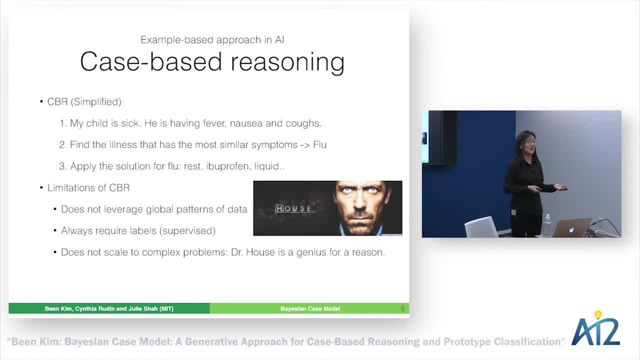 I don't know how many people watch Dr House. it's a medical drama, Okay good, So it's a medical drama. for those who haven't watched it, It's a medical drama about this genius doctor who can figure out mysterious. 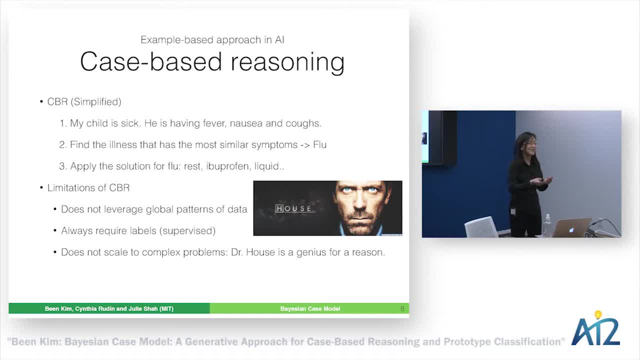 patients with mysterious symptoms and diseases and diagnose, find the right what's wrong with this patient And the solution space that Dr House is searching for is huge. It's a very complex domain, But this doctor is depicted as a genius for a reason. 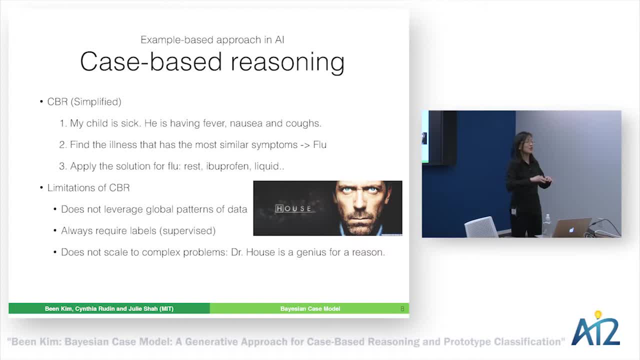 because normal humans are not really good at doing this. Matching when data becomes very high dimensional matching, and finding the closest solution and applying that solution closest and applying that solution to the newest incident. humans are not very good at it, And neither does CBR. 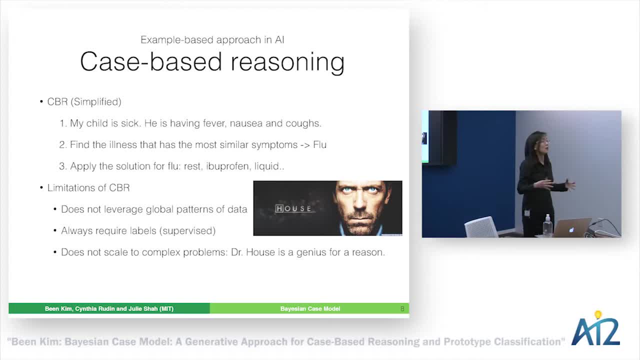 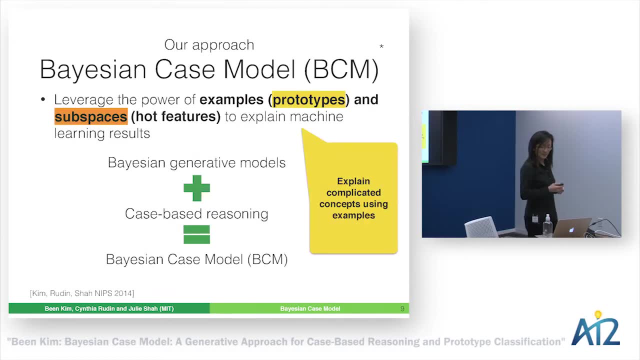 It quickly loses the intuition of power when it becomes a very complicated system, complicated data and complicated problems. Alright, so let me introduce our approach. We call it Bayesian case model. It is about leveraging power of prototypes, which are basically examples, and subspaces, which are basically hot features. 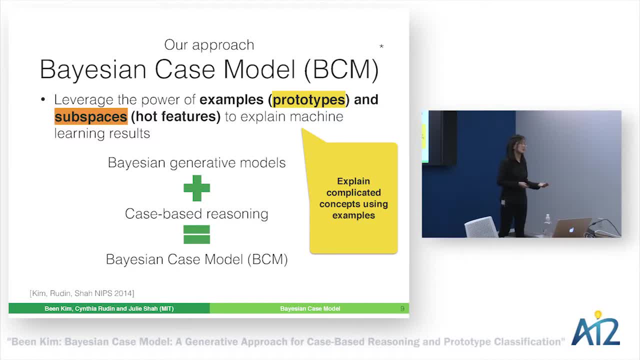 important features to explain machine learning results. So technically we combine Bayesian generative models with case-based reasoning and make Bayesian case model. These are just fancy way of saying we're trying to explain something complicated using examples, because we believe that's powerful. 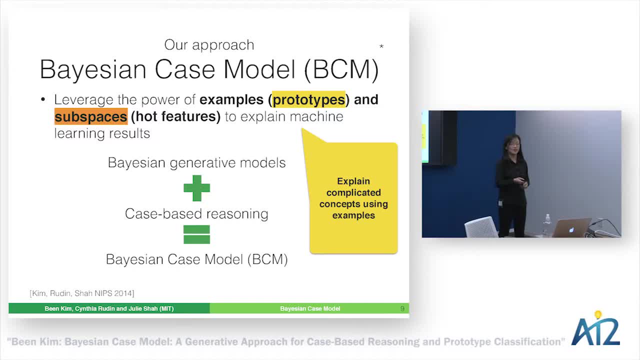 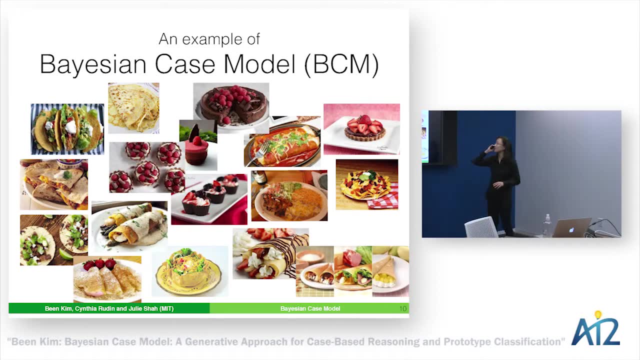 and that's just the way that humans think when they're making decisions. So before I jump right onto the model, let me give you an example, because I've been advocating examples, So I hope you're not too hungry because here are delicious looking. 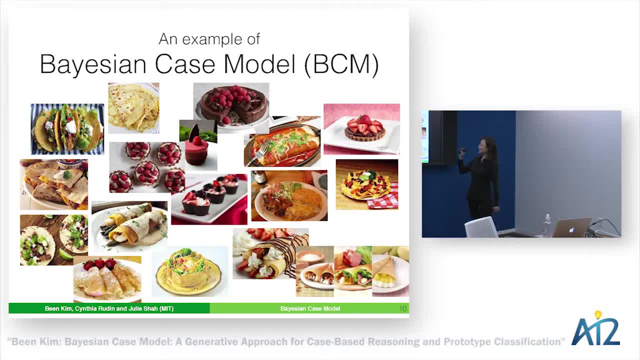 many, many dishes that I'm showing you. Can anyone identify clusters in these dishes? Mexican food and desserts. Good, yeah, these are all really good answers. There's one more cluster? Yeah, okay, well, you're really fast and you're really good at this. 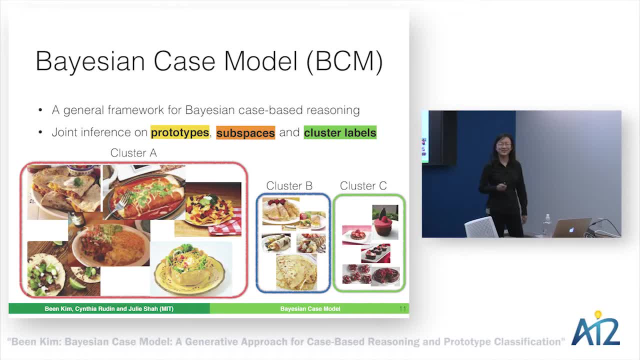 Okay, yes, so there are three clusters. You might be the fastest person. I've given up this talk a few times and no one gets it this fast, Amazing, amazing. So the first cluster is Mexican food. You see quesadilla, enchiladas, nachos. 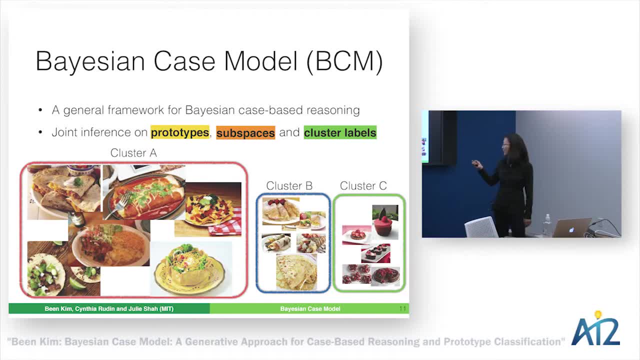 and salad, taco salad. And second cluster is the crepe cluster. It's got savory crepes and some sweet crepes and basic crepes. And the third cluster is desserts. In particular it has berry and chocolate, So Bayesian case model. 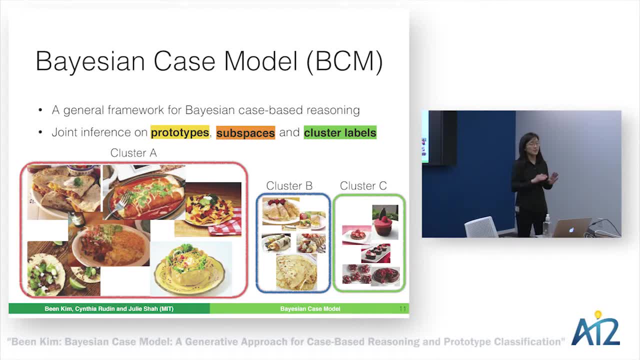 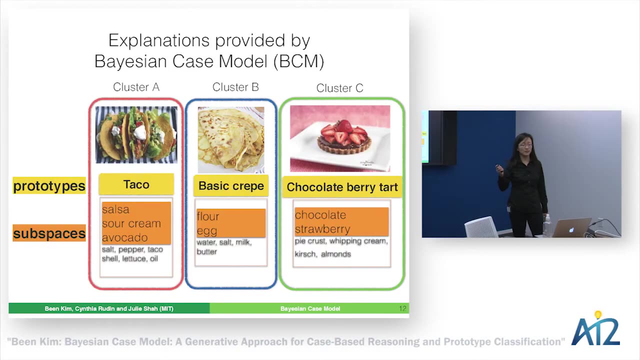 performs joint inference on explanations, which are prototypes, and subspaces, and cluster labels, which are these. So it's a clustering algorithm that also learns explanations at the same time. So these are cluster results. Let me show you how the explanation looks like. 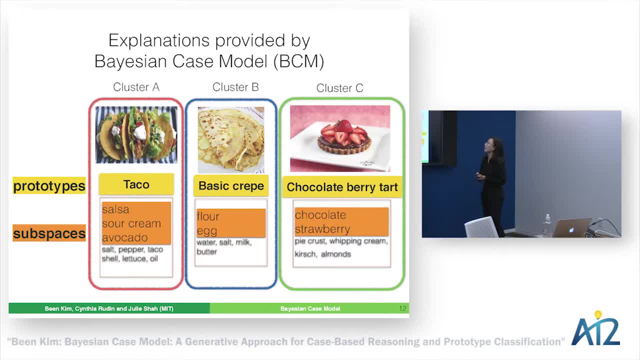 These are the explanations provided by Bayesian case model. First cluster is, like you said, Mexican food, But maybe someone. We happen to have an easy name for that cluster, Mexican food, But a lot of data points. we don't really have that easy name. 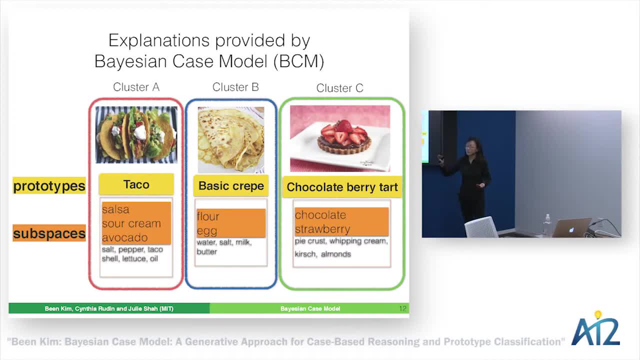 so we can quickly summarize that cluster. So what I can explain this cluster instead is by asking: oh, have you eaten tacos? If you've eaten tacos, the cluster A is like tacos. but the important features that you need to pay attention to. 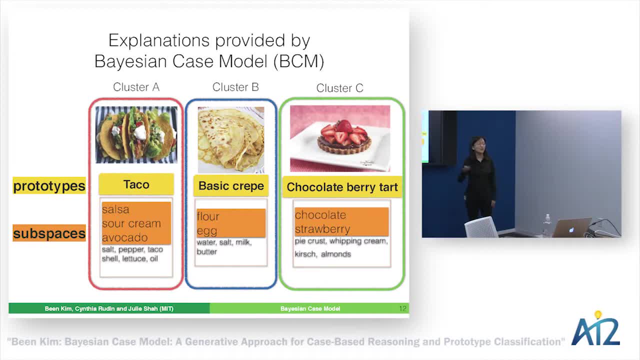 are salsa, sour cream and avocado. Second cluster is like basic crepe, but what important features are in that cluster are flour and eggs. And the third is chocolate berry tart cluster and chocolate strawberries are the important ingredients. So this orange marked. 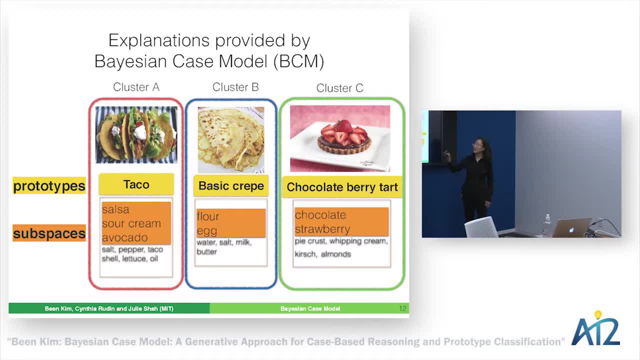 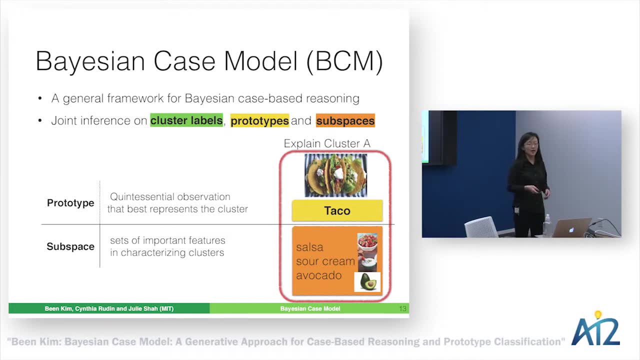 As orange. these are subspaces, the important hot features and these are the prototypes that we learned. So this is the way that BCM provides explanations. Technically, prototypes are defined as a quanta-essential observation that best represents the cluster. 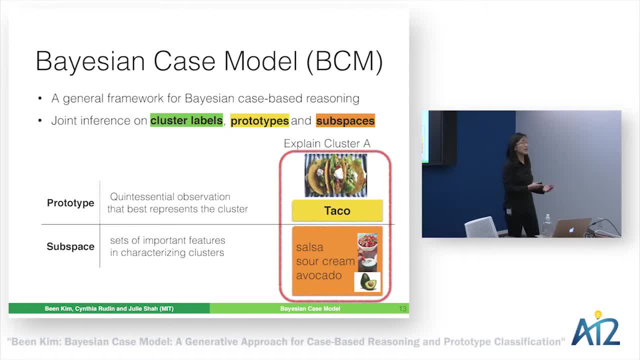 And subspace is a set of important features that characterizes, that characterizes the clusters. So let's go a little more in-depth of how this model works. I'm going to first explain how the clustering part works, but remember we're doing joint inference on everything. 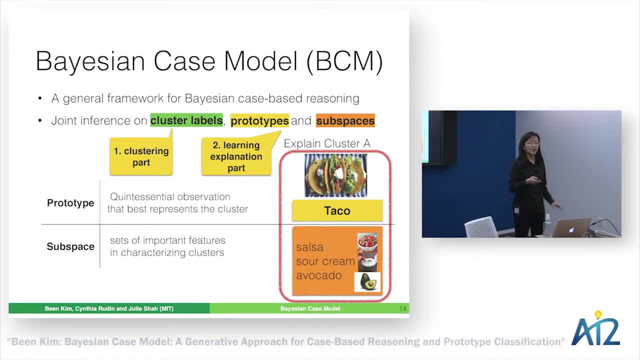 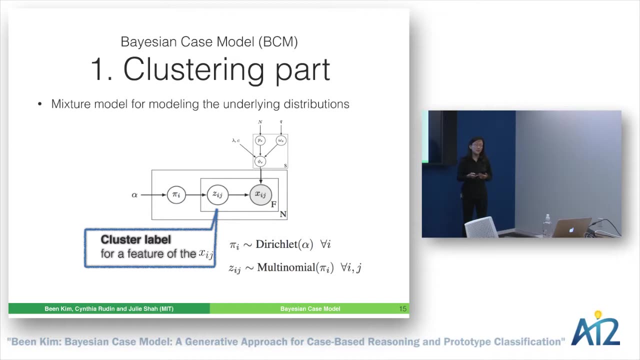 so these old three things happens at the same time. But let me just first talk about how the clustering part works and then I'm going to talk about how we're learning explanations. So first, clustering part: BCM leverages models. that is well-studied. 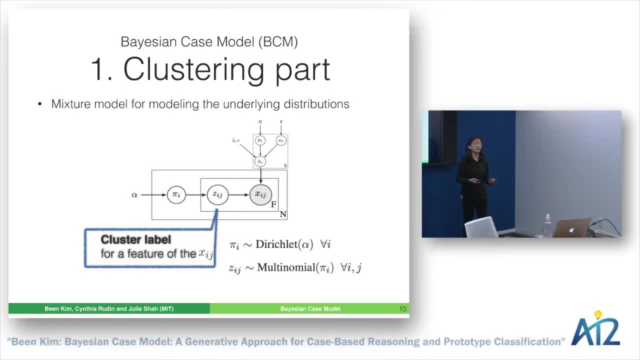 in Bayesian generative model community, which is a mixture model. Mixture model can is popular, has been very popular to model the underlying distribution because of its flexibility. In a short way of explaining mixture model is instead of When you have a data. 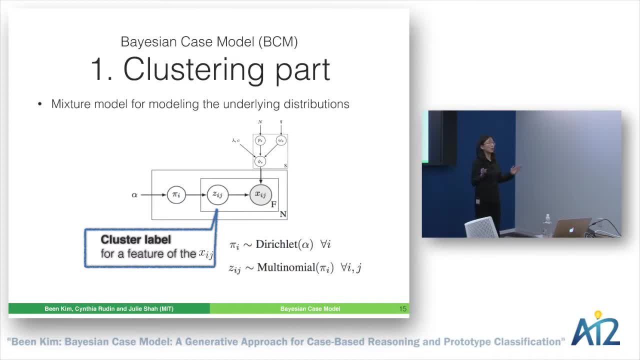 and you have multiple features for a data point, you're going to assign a label for each of these features instead of assigning one data to one cluster. boom and you're done So. that allows you a little more flexibility And this has been well-studied. 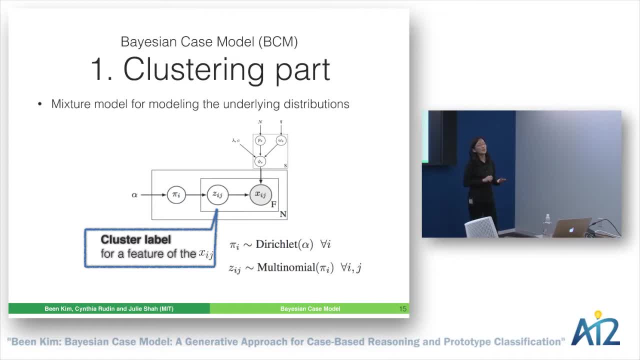 Lots of efficient inference algorithms have been developed to solve, to do the inference on the mixture model, such as LDA. Latin Dirichlet Allocation is one of the generative model that leverages the power of mixture model. Mathematically it's leveraging. 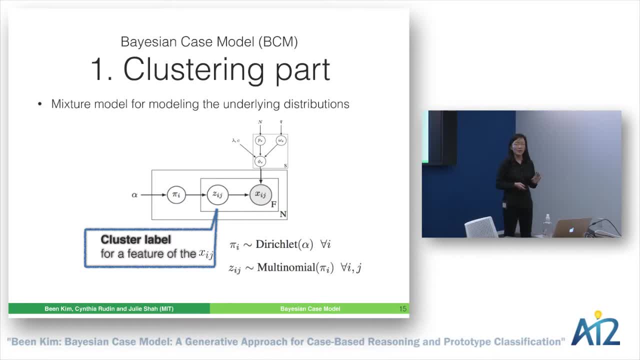 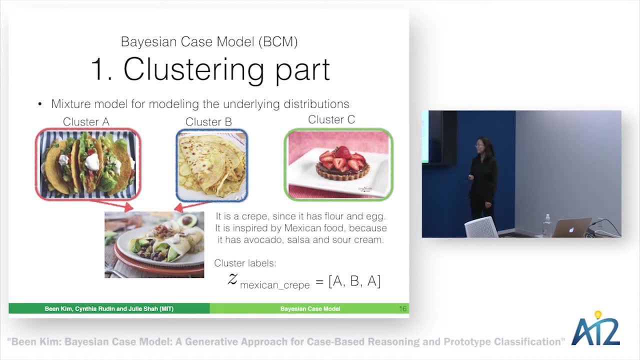 the power of conjugate, prior, multinomial and linear. So you can see here that we have a mixture model and a Dirichlet pair. But before that, let me give you an example of how a mixture model would look like in our running example of the recipe data. 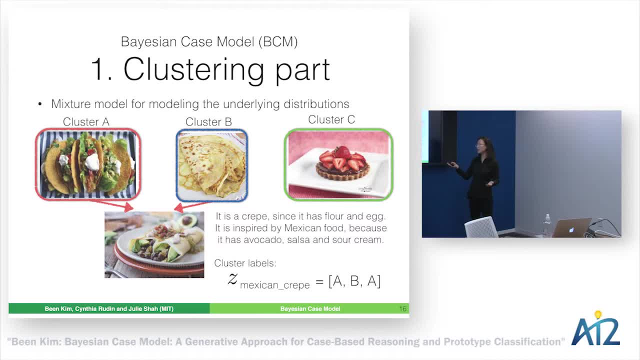 Let's say you have a crepe that is Mexican-inspired. You have some of the ingredients- avocado, salsa- but you have the crepe as a base. In this case, what a mixture model is going to do is label each of these features. 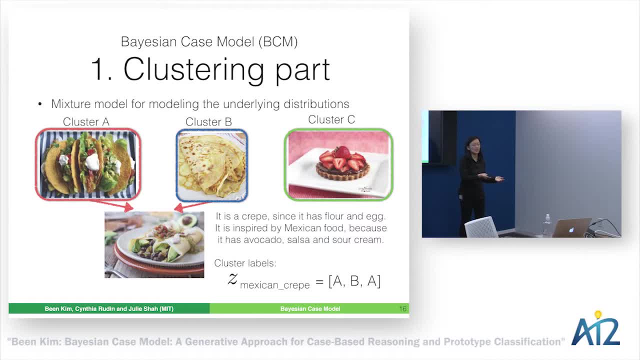 to and assign them to a different cluster, And salsa might be Cluster A- Mexican food- and the base crepe will be Cluster B, the crepe cluster, If you have a sweet crepe that happens to have a chocolate and berry in it. 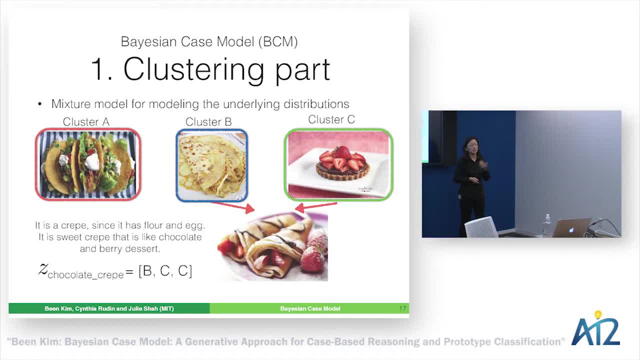 then it's going to assign some of the ingredients to Cluster C and some of the ingredients to Cluster B. So when you look at this one data point, you have some sort of distribution over clusters. So this guy has one B and two Cs. 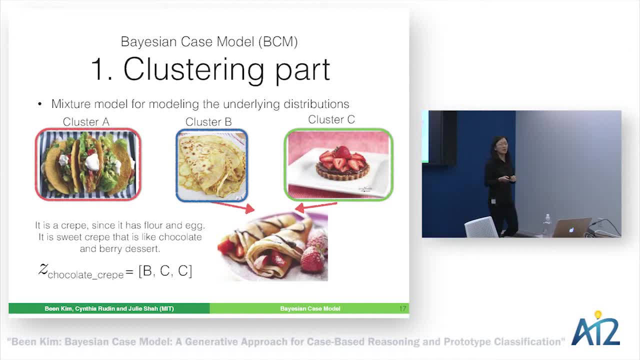 And this variable is explicitly modeled in the generative model and that's the pi variable: cluster distribution. So A data point is now not just A cluster but is a distribution over clusters, And this variable can be used to convert your clustering algorithm into classification method. 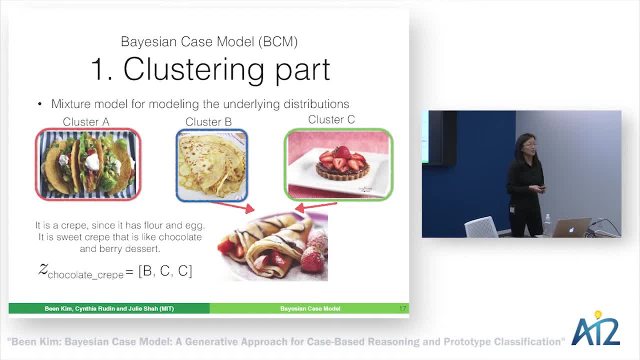 such that often used for evaluation. This type of evaluating these clustering models are firstly introduced by David Bly's first paper and original paper of LDA, So we're going to use this to compare our clustering model's performance with other models. Another thing that mixture model offers: 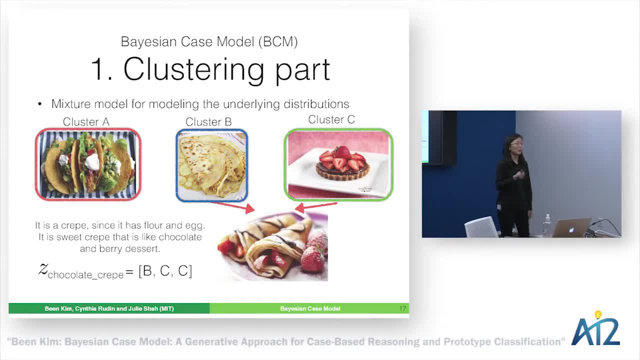 is this hyperparameter, alpha or any other name that you want to call this alpha to? What this alpha gives you is flexibility of deciding how many different clusters you want to have per data point. So, for example, in the previous example- maybe you want to see this- 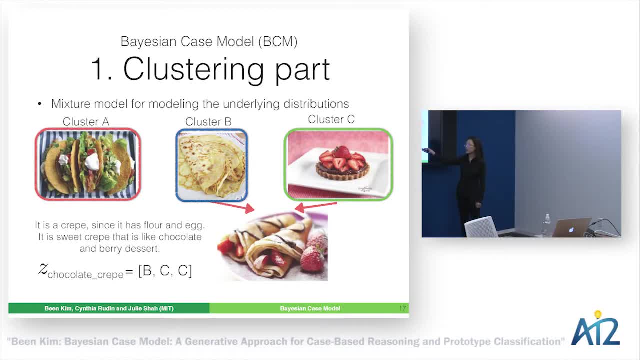 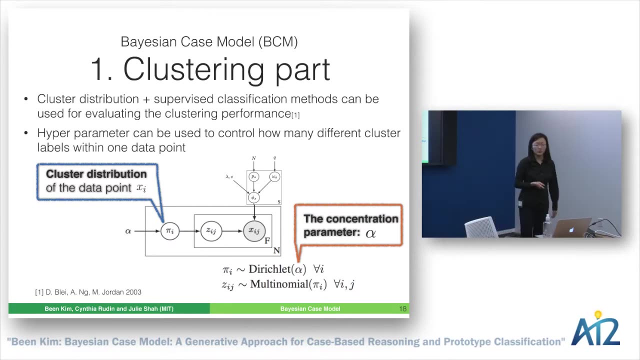 you just see this as a dessert and you want this data to be mostly really cluster C, Then you can change this hyperparameter alpha such that it would indirectly encourage that behavior. So that's the hyperparameter alpha that we have another control over. 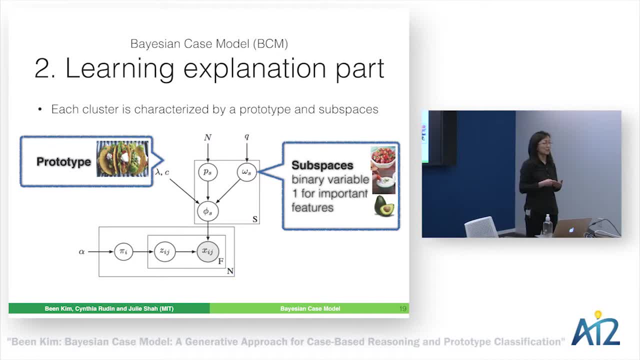 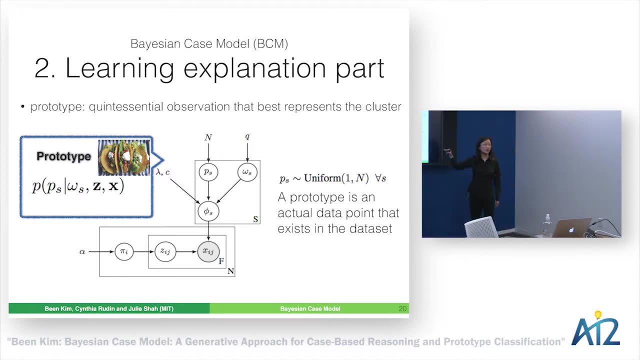 All right. so, moving on to the learning, the explanation part. The explanations are again represented as prototypes and subspaces. And let me first explain what are the prototypes. The prototypes are defined in our generative model, generative story. It's simply a uniform distribution. 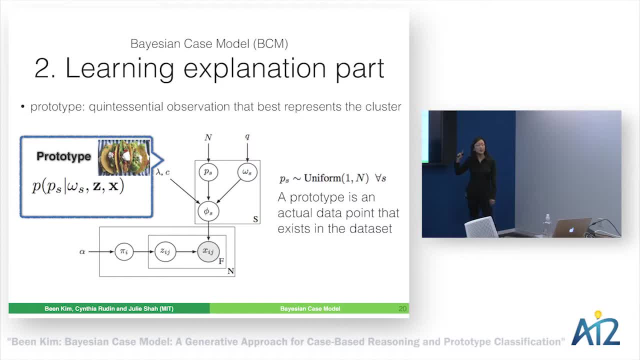 over all possible data points, And this is actually the key why BCM is intuitive. So, as compared to- as opposed to making a mock sample data point, something that didn't exist in your data data set, and making up and presenting it to the humans, 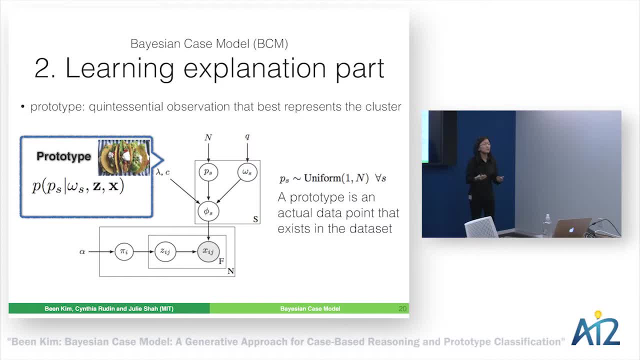 we actually select a data point that was given to us by the humans, So, for example, your disaster responders, I will, instead of making up an averaged cluster, case or incident, I will tell you: okay, well, cluster A is this case that you experienced. 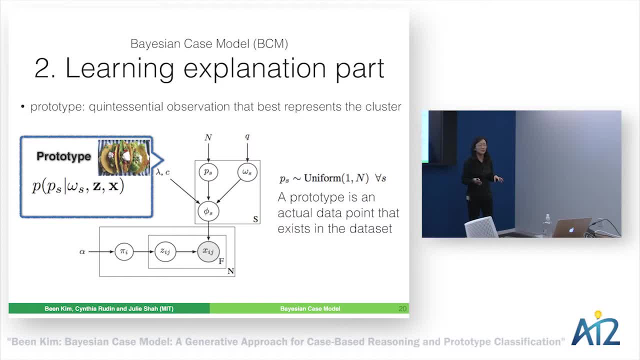 in 1996.. There's a high story, multi-story building, It was a high wind. And the human experts are like, oh yeah, okay, I remember that, I remember what the case was. And then I say, okay, well. 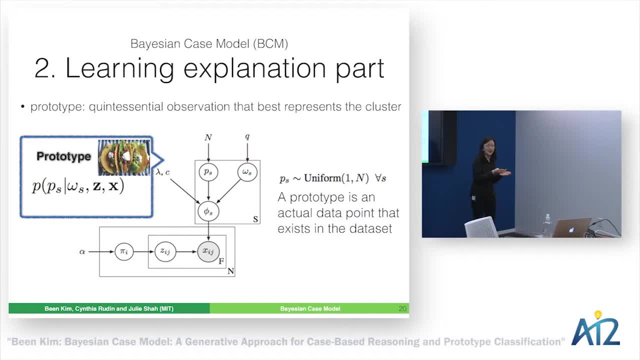 the cluster is. this cluster is about that incident that you had, but important features are this and that. So using the fact that we're using the actual data point is actually one of the key why BCM is intuitive. What's the part about? 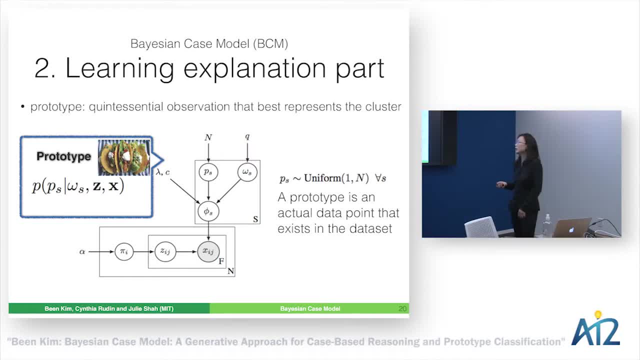 the uniform distribution. It simply models. you know we're not going to favor one data point over others when we're in the generative model story, But in the in the inference step, right, it will benefit, it will favor the ones. 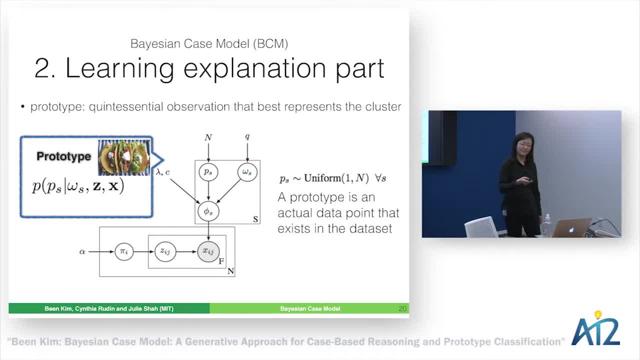 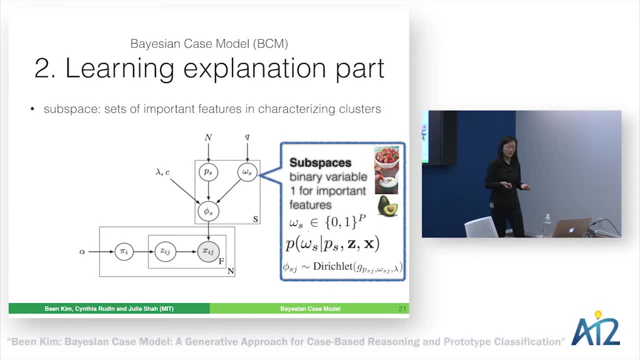 that better represents the cluster. So let's see. let's see how subspaces are learned and modeled. Subspaces are simply a binary variable: one for important features and zero for not important features. We decide to, we decided to incorporate the subspaces idea. 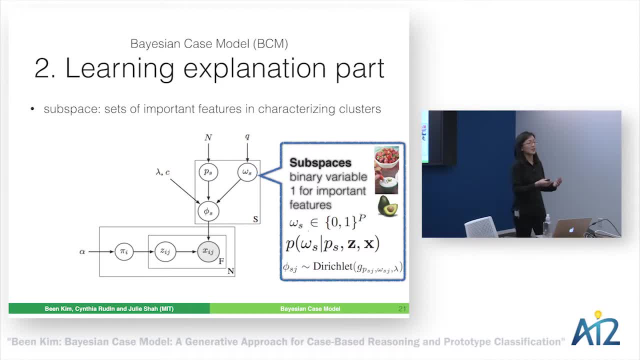 using the phi variable that explains the cluster. So the way that subspaces, this omega s, is incorporated into in the cluster in our model is using this g function, which I will explain very shortly, and making that g function to be a hyperparameter. 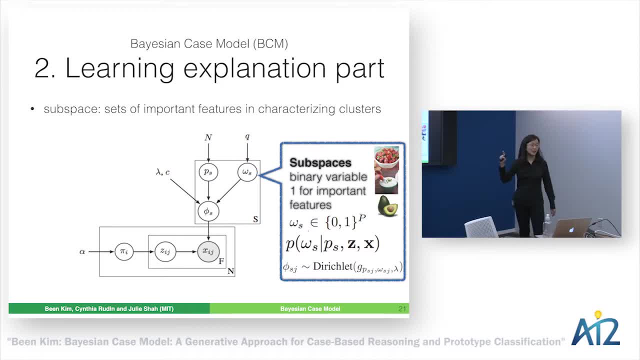 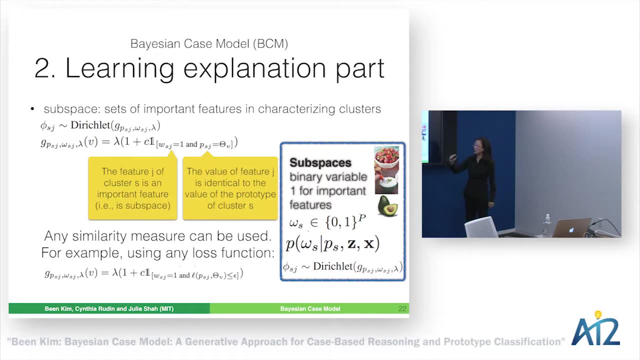 for Dirichlet distribution that phi is sampled from And phi is the variable that describes the cluster s. phi s describes the cluster cluster s. So let's look at what g function look like. So g function looks like this. It's a one way of describing. 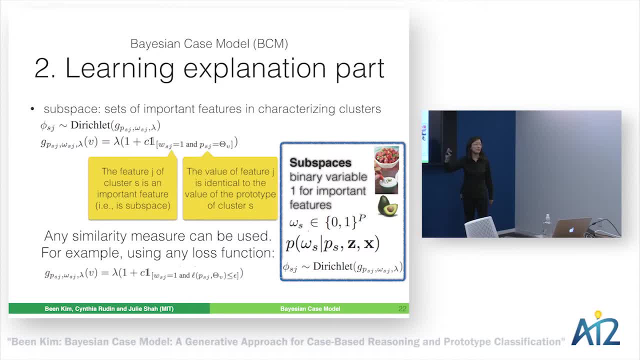 one way of defining g function. It looks complicated but it's really nothing but making. we're going to put same bump for all the possible features, except if that feature is important and you happen to have the same feature value as the prototype. 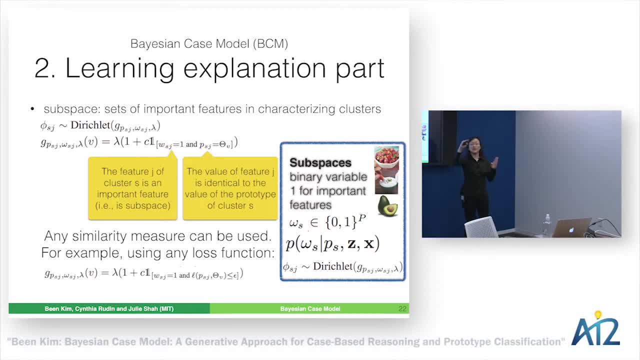 then we're going to raise the bump. So you're going to have something like this: if you have features that matches up with your prototype- So if you have a data point that is same feature value as your prototype, then it's just going to end up. 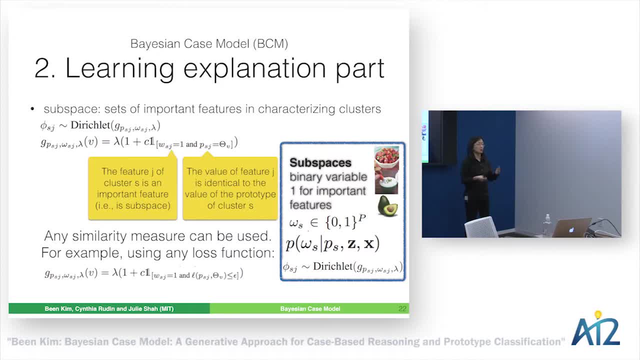 with a higher score And therefore in the Gibbs sampling step it will going to have a higher probability of getting sampled. And this is one way of defining function g. You can define this is a way of measuring the similarity, You can define this g function. 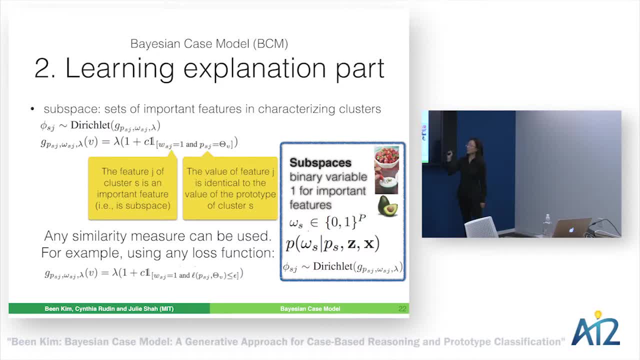 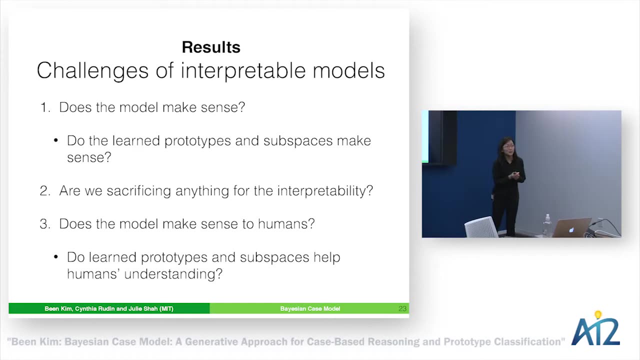 to be anything. You could, for example, incorporate a loss function or any other kernel, whichever you like- But this is the simplest form that we've picked up for this work. OK, So when I talk to people about interpretable models, 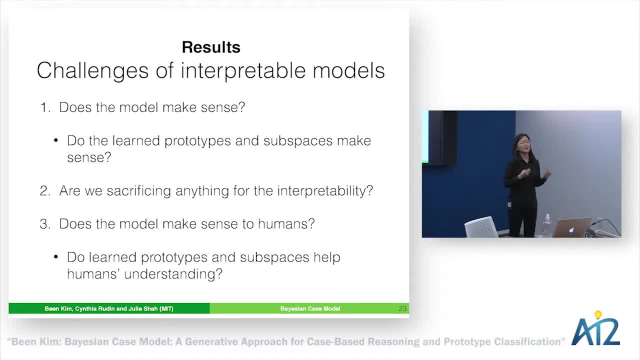 they have questions. It's not just about performance and predictability, It's also about a lot of other questions have to follow right. We have to show a lot of things. First thing to answer. the first question that I get is, before anything, 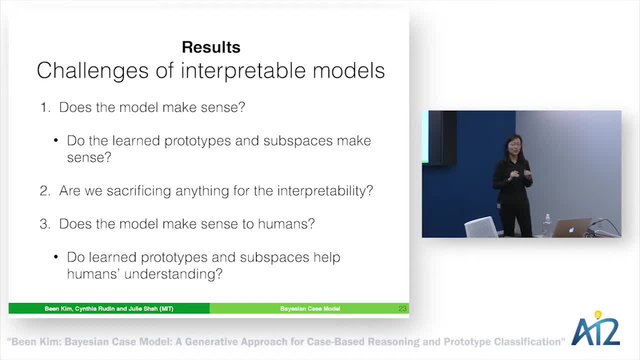 let's just make sure that this model you built makes sense. So you claim to learn these prototypes and subspaces. Does it actually make sense? Does it actually work? And then, once that's done, OK, well, interpretability is great. 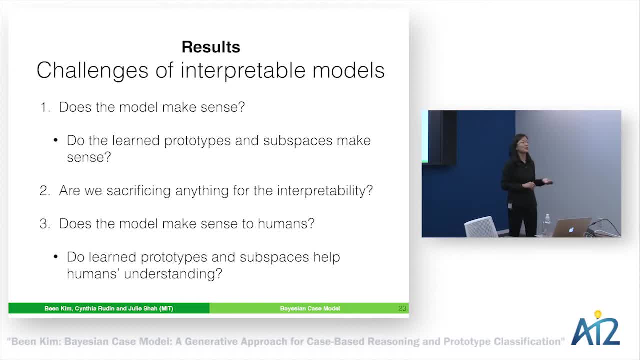 but what are we paying for? What are we sacrificing for this interpretability? And, lastly, does this really make sense to humans? Have you verified with actual humans that this thing actually makes sense to humans? So I'll show you answer these questions. 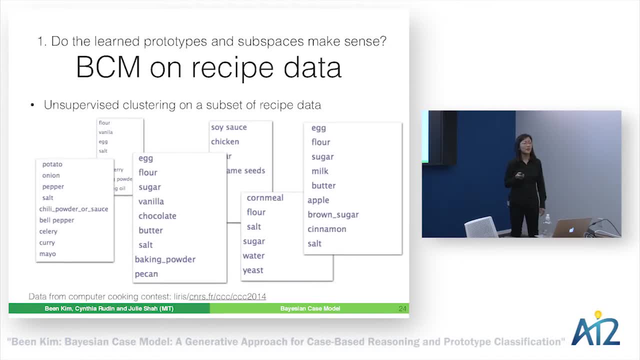 as a part of presenting the results. So first data set that we tried our BCM on is a recipe data. This is a publicly available data set. It's a part of a computer cooking contest data set where each data point consists of ingredients. 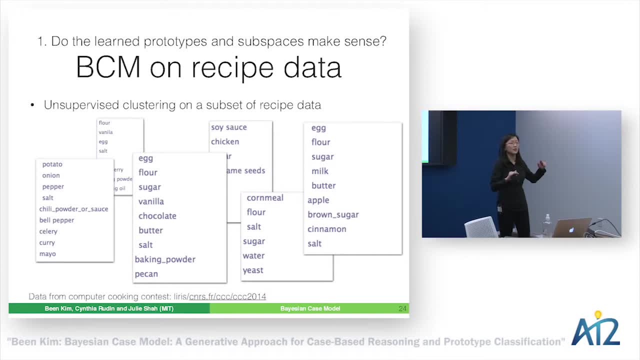 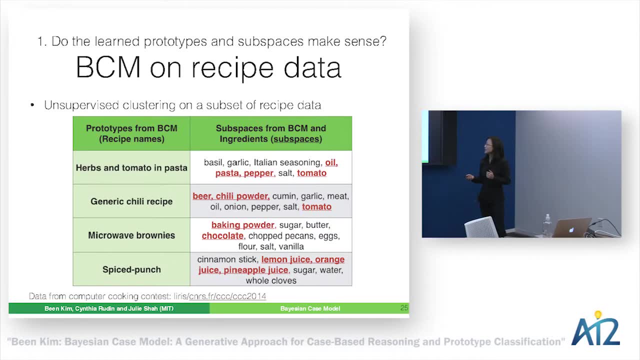 So it's a recipe data set, but the instructions of how to make the dish isn't there. It's just a list of ingredients And we ran BCM on this and this is what it learned. It learned for the cluster that looks like a pasta cluster. 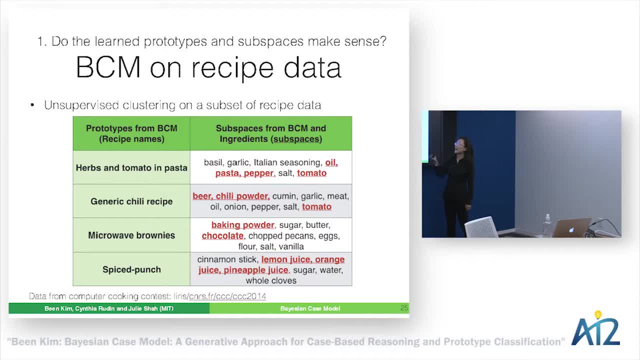 it selected that Irvine tomato in pasta is the prototypical dish of pasta cluster and it learned oil, pasta, pepper and tomato to be important features. the subspaces For the cluster that looks like chili cluster. it learned genetic chili recipe and selected beer chili powder. 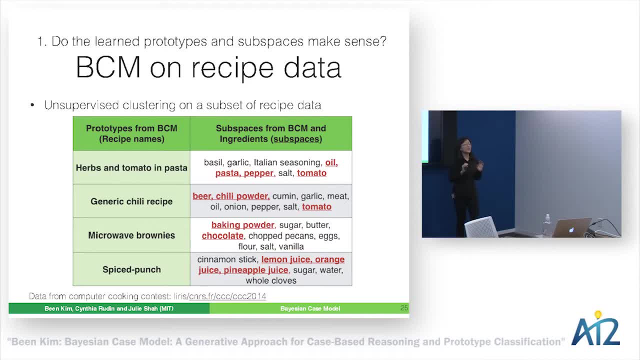 and tomato as subspaces. And if you're like my co-author who told me when I showed these results to her, she was like beer is weird. Beer shouldn't be in chili. Why is beer in chili? And I told her: 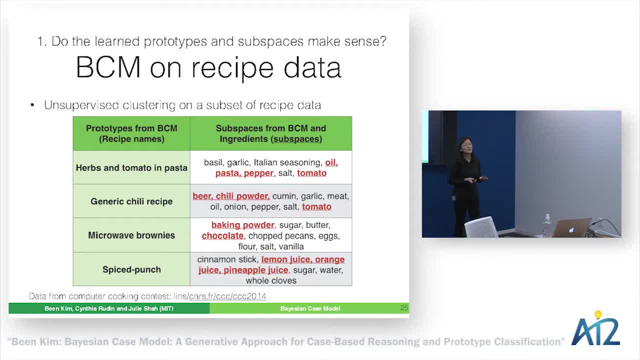 well, I mean, if you cooked chili, if you haven't been putting beer in your chili, you should. It makes a lot of difference. So beer is there, You should. Beer is a great ingredient for pretty much any dish, really. 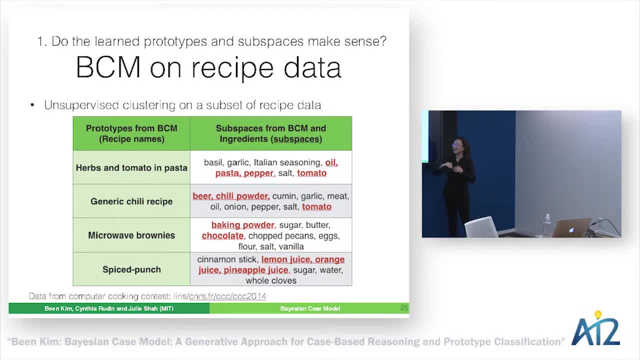 Microwave brownies are selected as the prototypical dish for the brownie cluster, and it learned baking powder and chocolate as subspaces. Punch cluster was an interesting one because it has such a variety of ingredients. when you're making punch, BCM was learning at each. 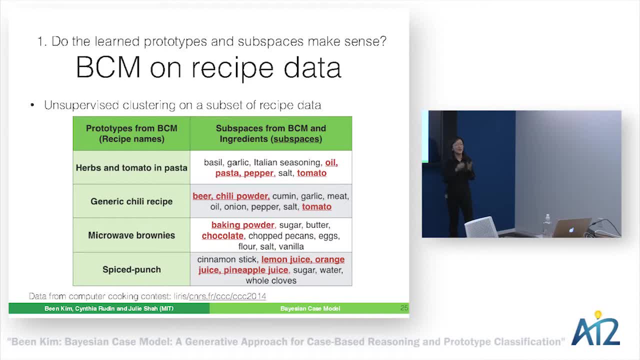 well, I'm doing Gibbs sampling to jump a few slides ahead. I'm doing Gibbs sampling and each Gibbs sampling. there are a lot of modes to jumping back and forth from, But what BCM settled on is what to me looks reasonable. 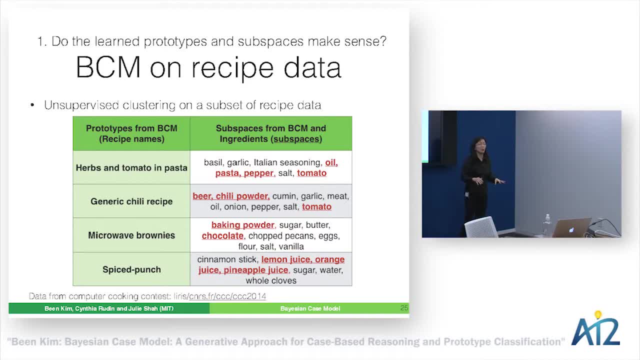 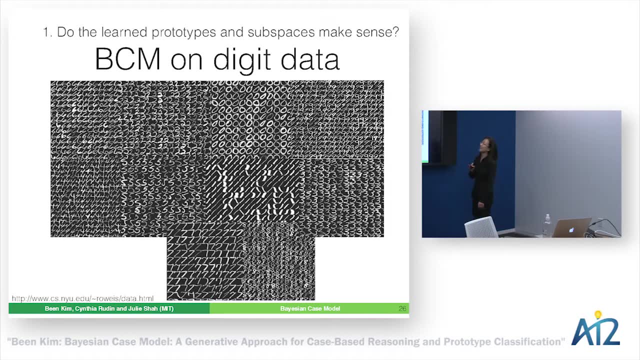 It picked up juices, the base ingredient for punch dishes. All right, So second data set that I ran BCM on is handwritten digital. yeah, Where are the? I mean you showed four clusters. Are they exhaustive or like these are four? 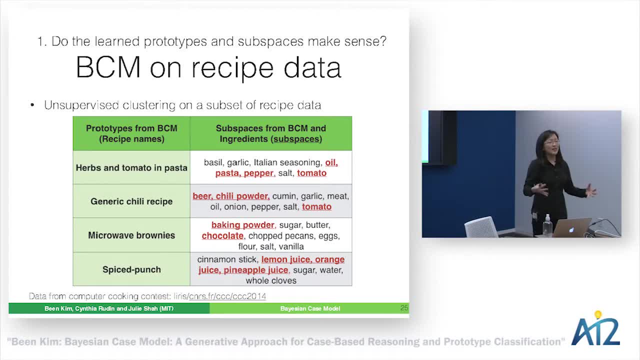 of the many clusters you have? That's a good question. So we selected the recipes that we know we might be able to identify. Remember, this is a clustering algorithm, right? So when the results are there, we don't have a ground truth. 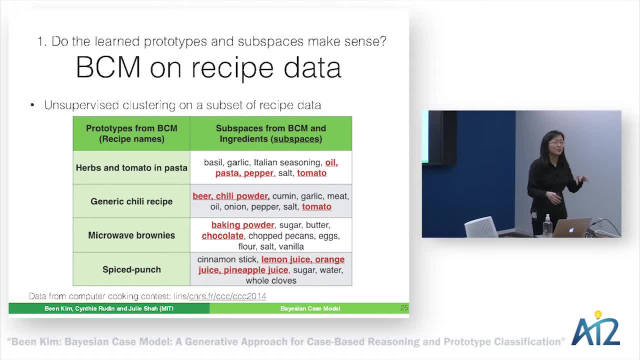 of like: what is this cluster? right? You might put, say, pasta and pizza cluster together because they're similar compared to other data points that we had in the data set. So what we did is that we collected the subset of this recipe data set. 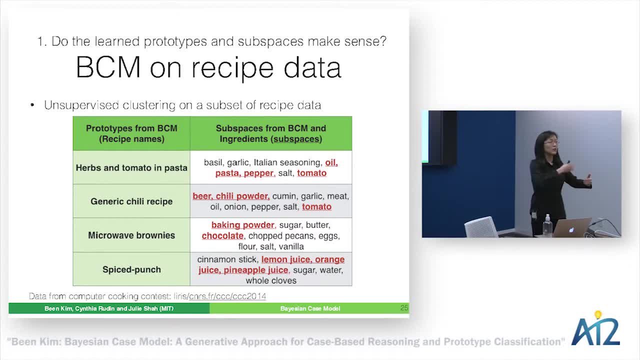 that we know that there are. when BCM learns something, we can identify each cluster what that is, and then I'm showing you there, showing those four clusters here I'm wondering why, like tomato, is picked up as an important feature. 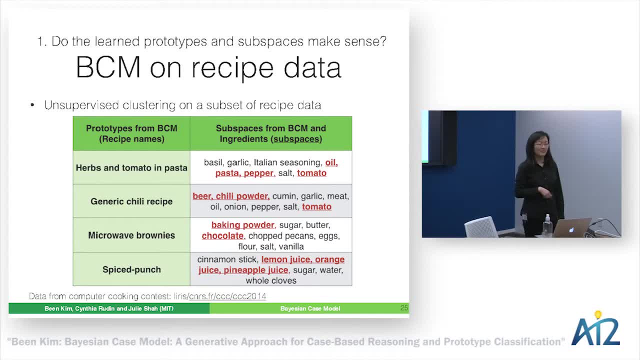 while salt is not. I don't see salt in brownies or punch. Yes, Salt is not picked as a Yeah, So what It actually- that's the right thing that BCM did- is salt. it did not pick the salt because, if you look at it, 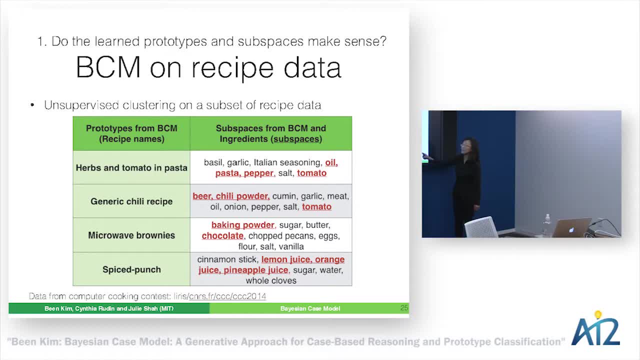 salt is everywhere. right, Salt is here. salt is there. salt is there. No, that's not it. Right, Oh, it's there. Yeah, yeah, So it's kind of common ingredient across the cluster, so it shouldn't pick it. 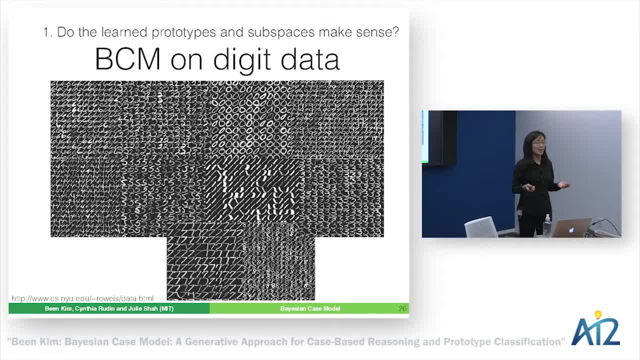 So we also ran BCM on a handwritten digit data set and this is a digitally written data set. This is a pretty widely used data set by Provided by Sam Ruiz in his website. It's It's digitally written, so, which is why. 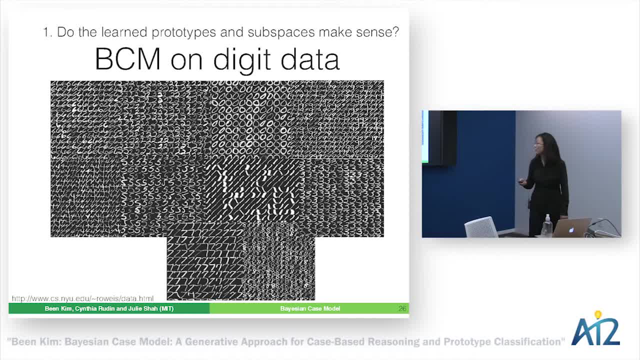 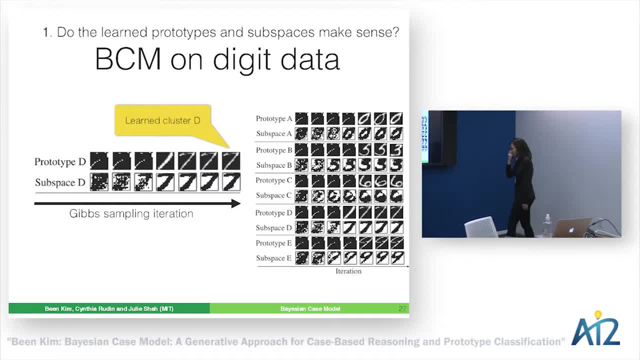 it's white and black are flipped. So these are zero and other Zero digits from zero to nine, And this is the results when we ran BCM. I'm showing you as the Gibbs sampling iteration goes, So in case you're not familiar with the Gibbs sampling. 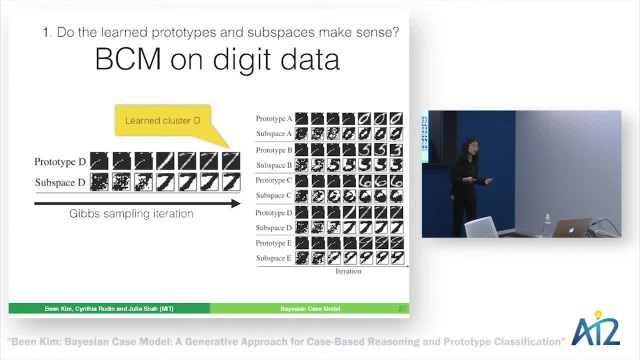 what you want to see. it's an iterative method to find a good solution, So you're doing some sort of random walk in the solution space. So what you would like to see if it's working as you go from left to right. 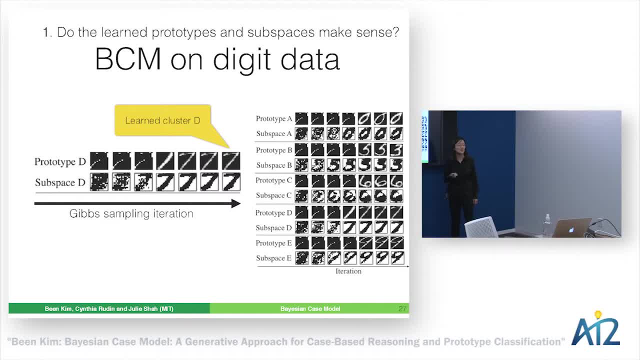 you want the right solutions to be better looking than the left ones. So the first cluster A looks like it's learning digit zero, this one three and a little confused with five and six and seven and nine, And what we used is the dumbest possible feature. 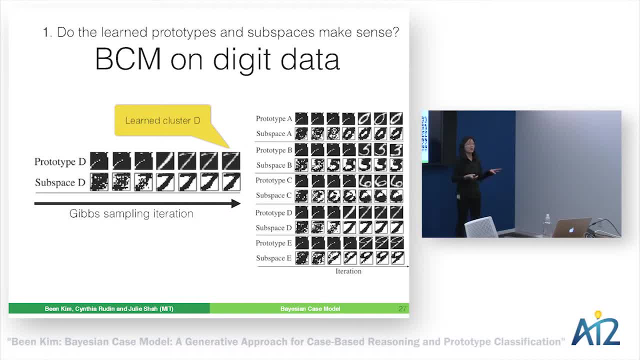 for this handwritten data set. And when you do that, other literature also shows that three and five were Irving confused. The feature we use is just 16 by 16. We flatten out into this vector 256 vector and just use that as a feature. 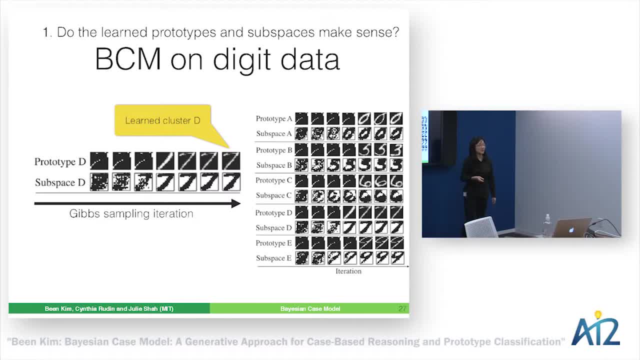 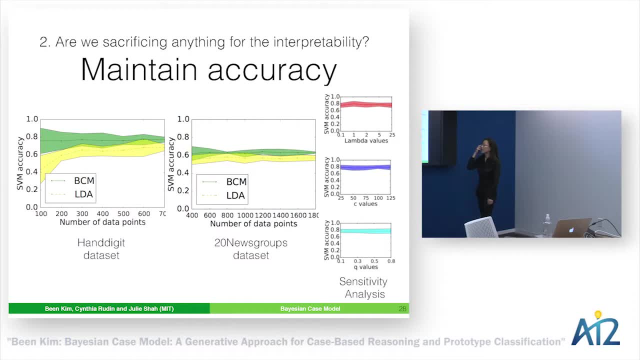 And when you do that, this is actually pretty common mistake that made when you use this data set. So we also see that here. All right, So hope I convinced you that the prototypes and subspaces that BCM learned is reasonable. Yeah, So I thought. 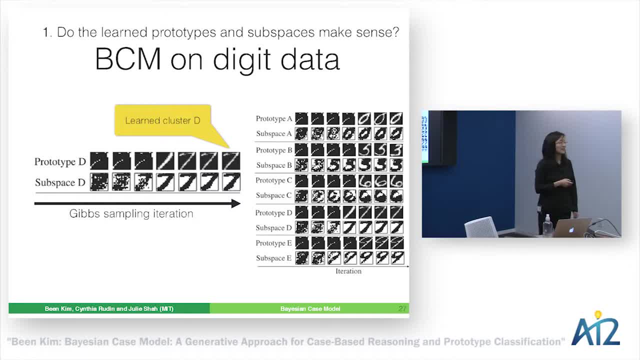 I understood the prototype was a specific example. Yes, It looks there like the prototype is evolving, So in your generation. Yeah, So this, each black boxes, are one data point. These, each is one data point. This is a data point. This is a data point. 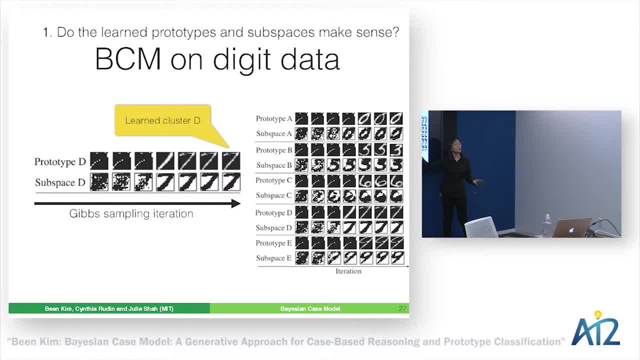 But it's not evolving, It's. I'm showing you a data point at each Gibbs sampling iterations. So basically, somebody wrote up really weird early on, Yes, And I verified. actually it really puzzled me, So I verified and this is there. 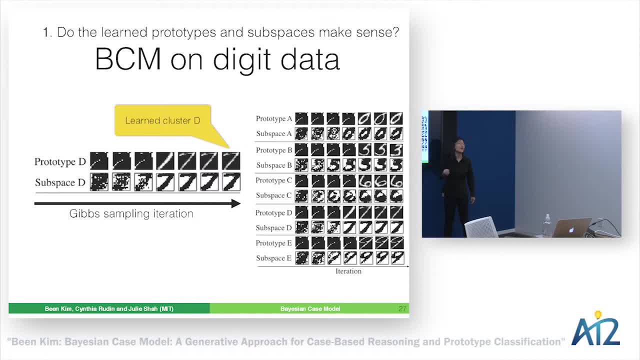 So that is an example. Yeah, It's an example. This is an example. Yeah, Oh, I see That's what confused you. Yes, And these are also, yeah, Very popular example. Yeah, On the previous slide where you had the recipes. 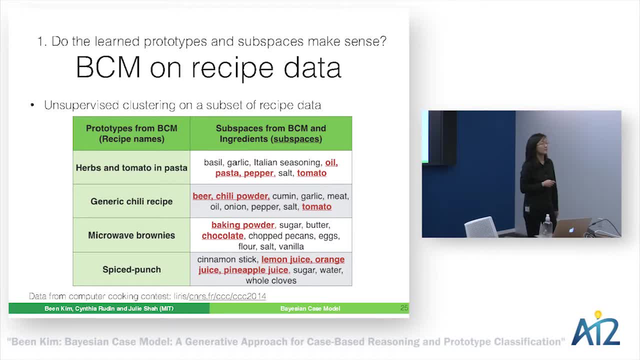 is that? yeah, this one, And it reminded me of how this is different from just doing clustering with PCA or something like that, And wouldn't you get the right components and the clusters? Or are these also particular examples I see? So PCA wouldn't. 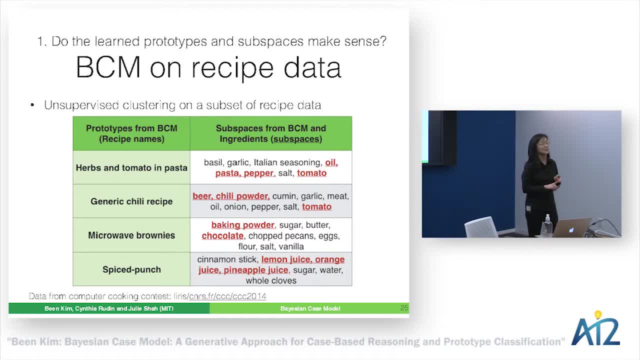 it would get you a linear combination of features right, So it wouldn't give you the subspaces, for example, And it would actually. it's not. it would try. it would make sure that all the features that you're in a combination. 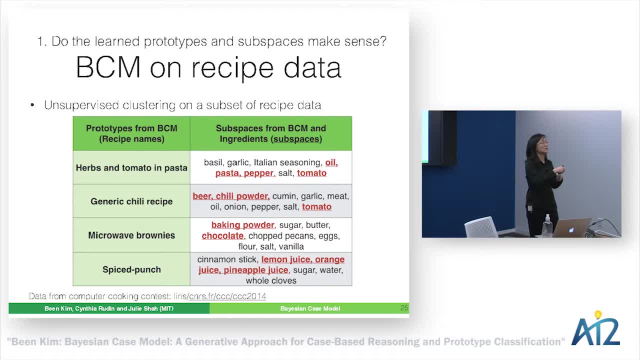 are orthogonal, which means that each feature that you get, even if you pick the largest coefficient feature, you're probably not going to get the same solution, Although I haven't verified it personally, But it's a very different sort of approach. 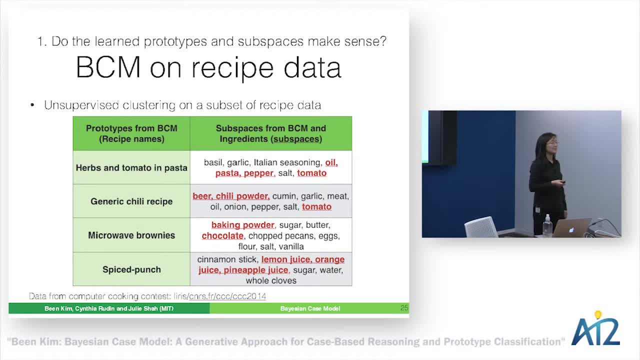 Does that answer your question? So, definitely. so you're going for not necessarily low rank, but sparse, Yes, Sparse and representative, Yeah. So, going back to the digit example: Yeah, It seems. or one more slide actually: Yeah, So it seems like. 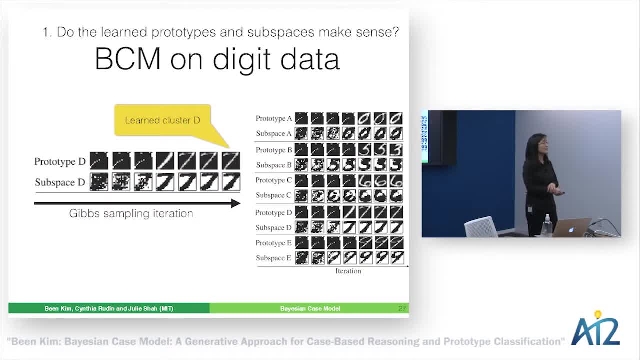 it's easy to kind of look at that subspace because of the features you chose, Right, But does it? does your method depend on kind of the feature space to be able to choose features that you know enable exploitability? This is a great question. 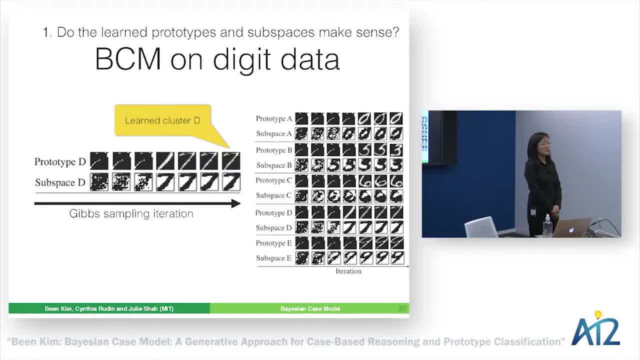 So, yes, So my method assumes that the features, whatever data that you gave me, those features that you gave me, are actually features that make sense to you. So the example that may not make sense, well, maybe, maybe it does. It does. 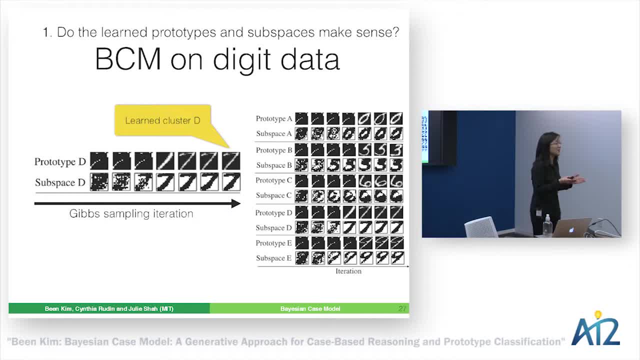 may not make sense. is maybe audio clips in the like frequency domain Right, If that's your feature, hopefully that makes sense to you. If that doesn't make sense to you, that's the subspaces that BCM will provide it to you. 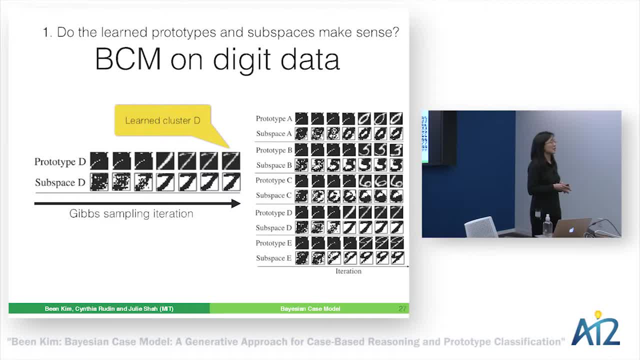 So, yes, that's an assumption that we make, that features that were given to us should make sense to at least like you to you. So the way the features were fed to your algorithm was a 256 dimensional vector. So if we listed those, 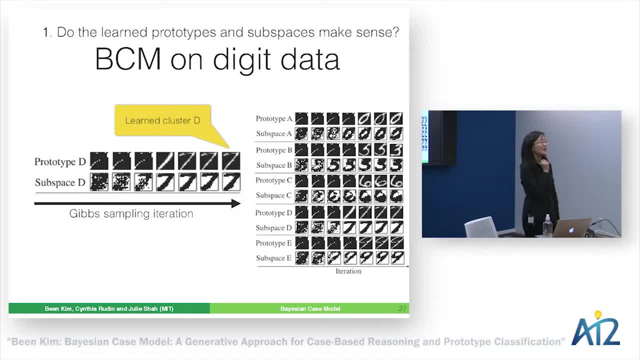 as our. that picture would not have made any sense to humans because you relayed it back out in the original picture form. True, Yes, true. So yeah, if we do some feature transformation and then that's the subspace we learn. 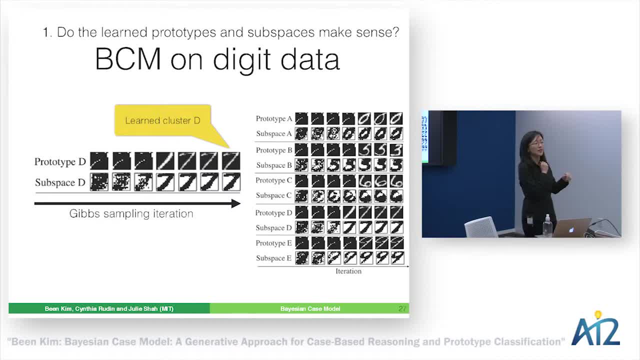 then that would also be a problem, Unless we invert it back, and that still makes sense, right? Yeah? So you were saying you picked the examples for the recipe. for the first case, did you pick a balanced number of recipes for each of the categories? 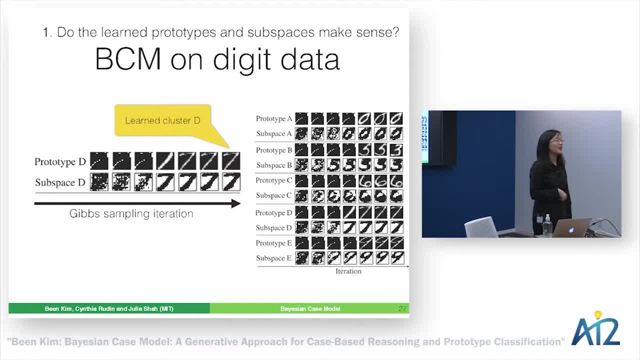 I see. Yes, I made sure that they're roughly in the same number, because otherwise it's going to be difficult. Okay, I guess that's. my next question is: how do you handle cases where, like one of the classic examples we will study in clusters? 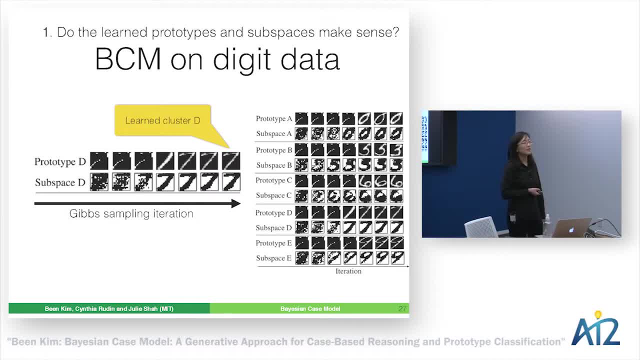 is how to put cluster color space into color names. It's been studied since the 1960s and, like we have a very defined concept of red, whereas green and blue right, right, right, right right, So that will be a very common problem. 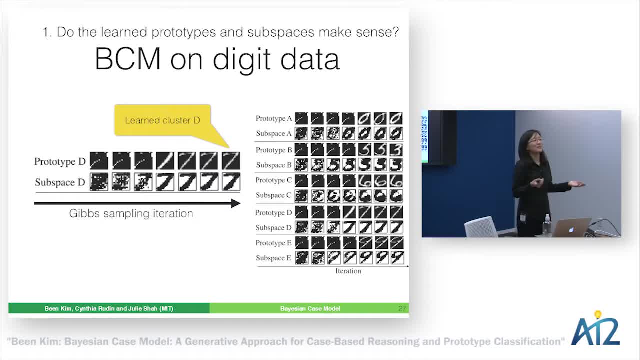 for any clustering algorithms, right Gaussian mixture model. if two means of these clusters are similar, then. But in real world a lot of the clusters are not balanced. and how do you- I see If like imbalanced data set, how would you do it? 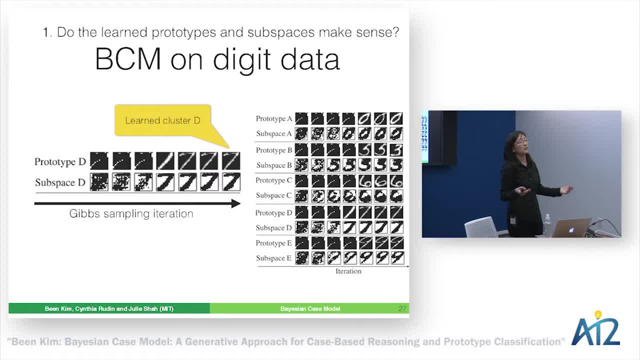 I see That's a good question. So for mixture models it relies on data points being. it's not particular for the BCM model, but any models that using a mixture model or any kind of naive feature space modeling would have the same problem of what you're describing. 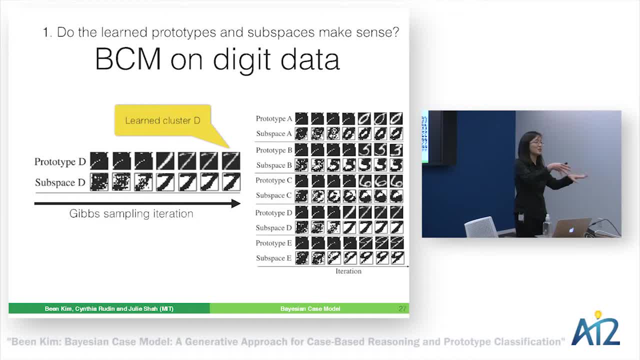 If features, data points are right next to each other, on the top of each other, then there's no way for us to distinguish. It would need extra work to transfer those features to be more distinguishable, or some other method. There would be something perhaps more fundamental. 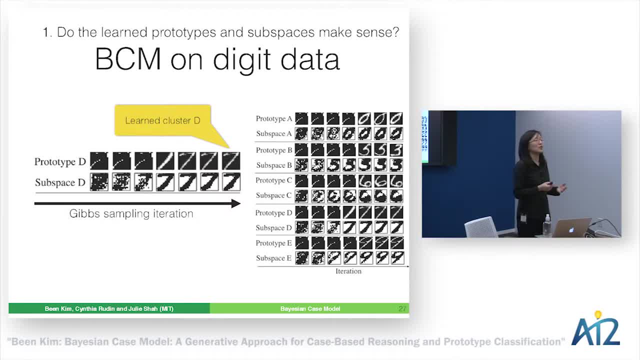 to clustering method in general than it is to you know. But that's a good point. If we could kind of map that current naive features to a higher dimension and keep the intuition and make it still understandable, that would be. that would be really good. 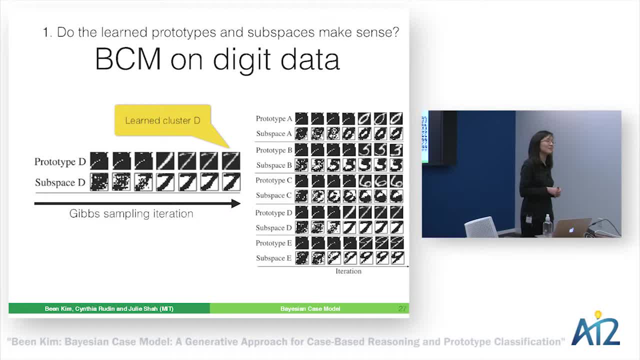 Yeah, I guess the related question is some things like, for example, when people pick a photo type to represent a particular color. almost everybody in the world- people survey this from like 110 different societies- pick the same red, but people actually pick very different blues. Oh, interesting. 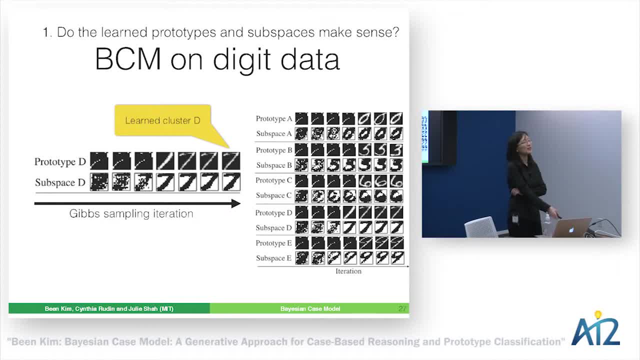 How do you deal with that? So that example that you gave me is how people perceive clusters to be different depending on the culture. I see, Or just like in some clusters, the photo type may not be so good for some people, Or people agree. 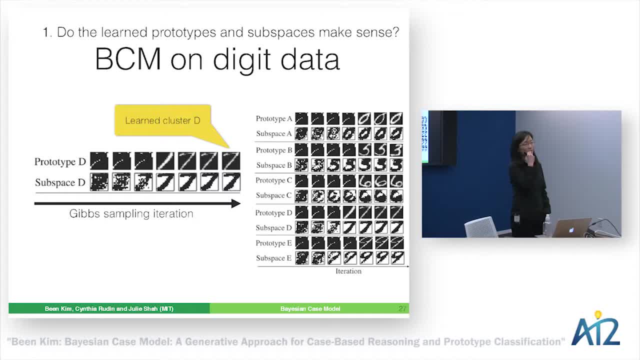 on multiple photo types. Oh interesting, Oh interesting, I see. So, if Right. So in your example, we want kind of have multiple prototypes for the blue and you agree on the prototype? Hmm, Yeah, yeah, yeah. So let's see. 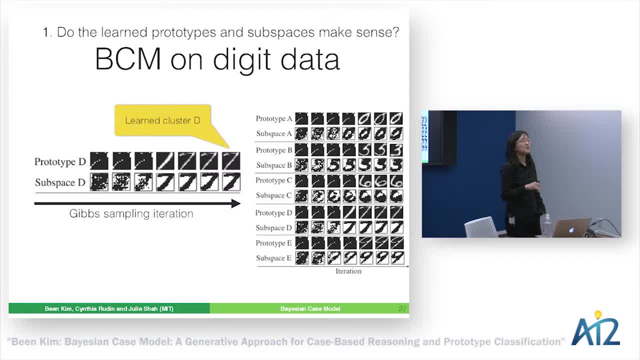 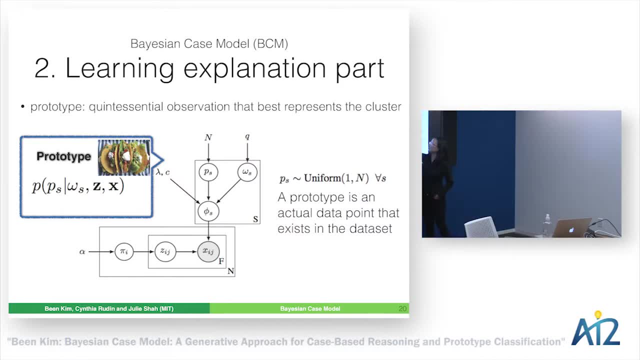 I can think of very simple extension of the BCM to make that happen. So you basically would need another box on the top of my model here, right here, to learn multiple prototypes And if that's the case, and maybe we could automatically also learn number of prototypes. 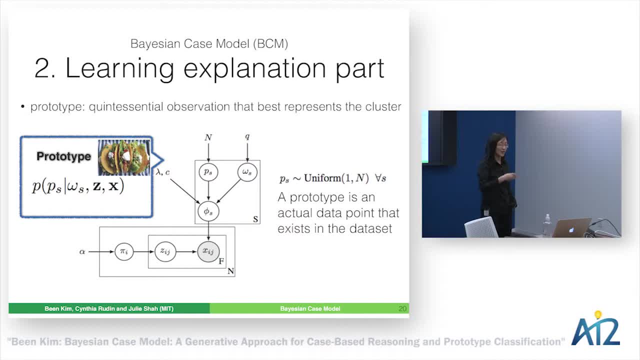 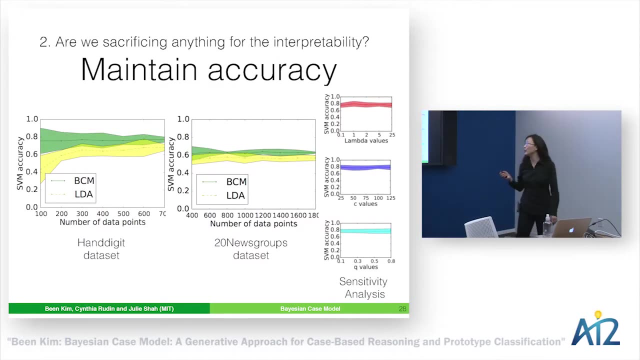 that is mixed, and you can put a non-Basian, non-parametric Basian in these restaurant processes- fancy prior to do that. But yeah, that's an extension, that's possible and it's a good point. Great, Okay, So I think. 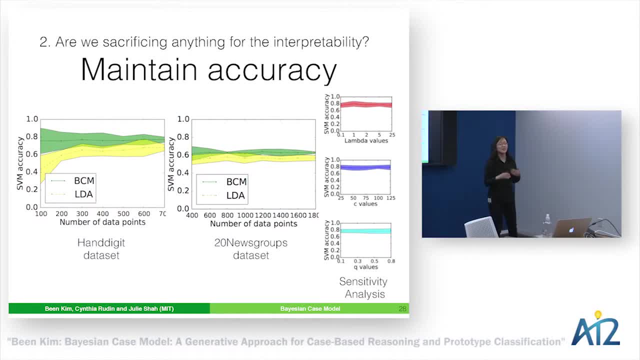 I was here, Yeah. So the next question that people ask is: okay, well, interpretability is great, It's great if we have it, but what are we? What's the cost? We show that BCM maintains accuracy. In fact, BCM beats. 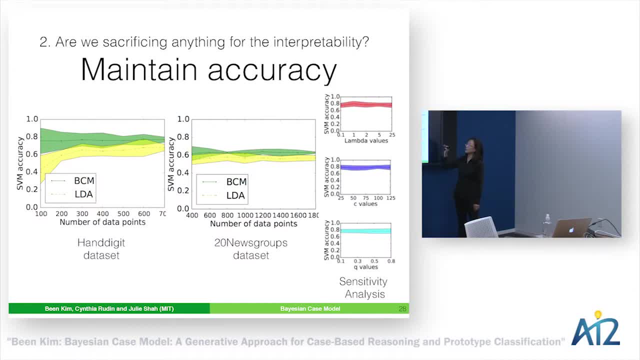 many of the settings that we tested. The green ones are the BCM, The yellows are the LDA. So the way that I evaluate this is- again in a few slides back- using the cluster distribution and you combine that with SVM to get the classification. 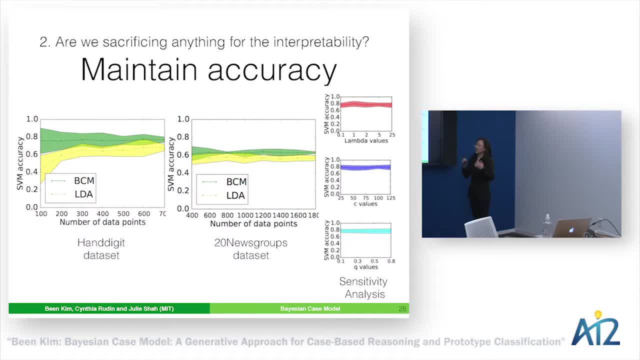 accuracy. So we show that and that's great. We also did sensitivity analysis. This is basically: we have some hyperparameters in BCM. If we change them a little bit does it make dramatic difference in our classification accuracy? And we show that for a number of. 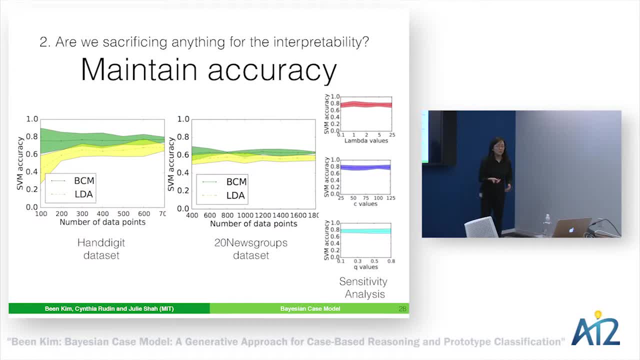 For all the values. it does not. So that shows us, yeah, we don't have to worry too much about the hyperparameter values, as long as we set them in a reasonable range. reasonable range defined over here, it will. It's pretty robust. 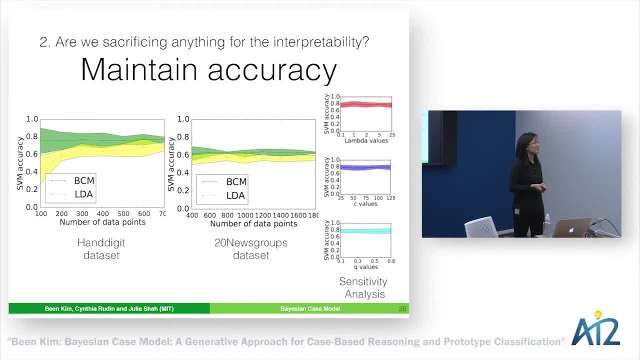 to that And that's a function of the amount of training data you have there, right, Some parameters yes, some parameters are no. yeah, So, for example, bumps like the, the g function bumps, how, how we are going to score the similarity. 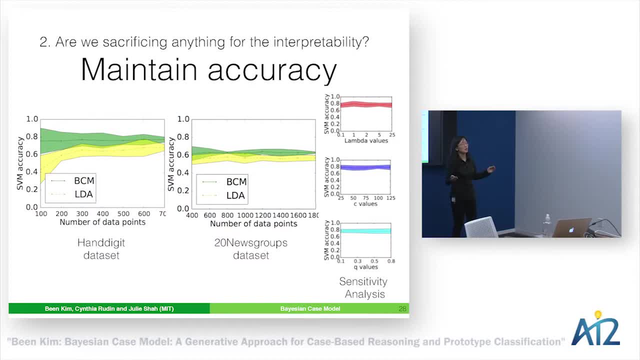 between data points and your prototype. Those bumps are not relative to your- your number of data points- But the, the pseudo counts for Dirichlet hyperparameters like alpha or other parameters that relate to those Dirichlet. that's a pseudo count for your data set. 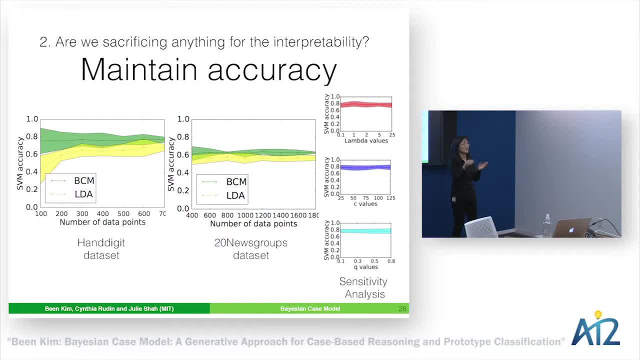 and it will be directly added onto. if you compare your data set with the number of data points, it will be directly added onto your data set, right? So that will have relation with the number of data points. So is this a lucky coincidence? 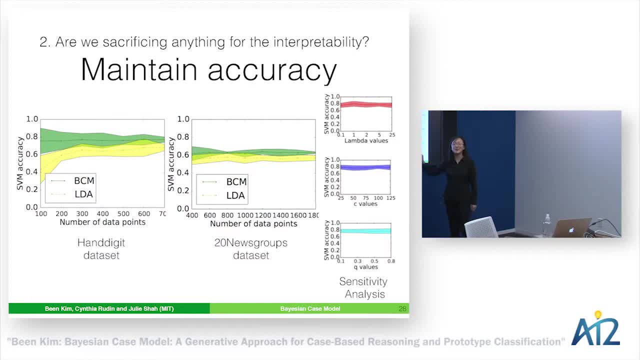 or is there an upper area reason to believe that BCM will outperform LDA? This is a really good question, because it really puzzled me when I first got this like why is it doing better? That's weird. So perhaps BCM is a. 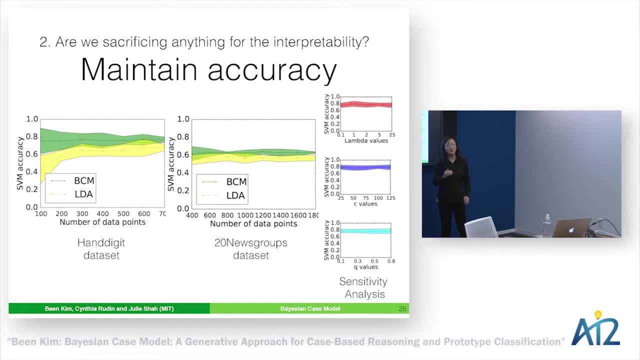 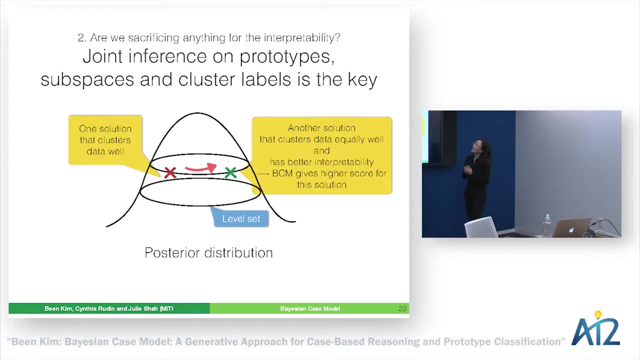 smart regularizer that acts on the solution space, that pushes the solution into a better space, that does not overfit the data. That's one explanation, All right, So it's a good segue for my next slide. So we wondered: why is this happening? 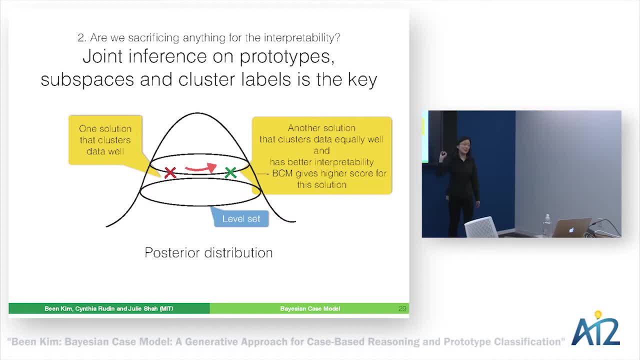 and this is a graphical explanation of why this might be happening. Think about a posterior distribution from and a level set in that posterior distribution represents all the solutions that are equally good in terms of clustering What we think that BCM is encouraging, the solution, the Gibbs sampling. 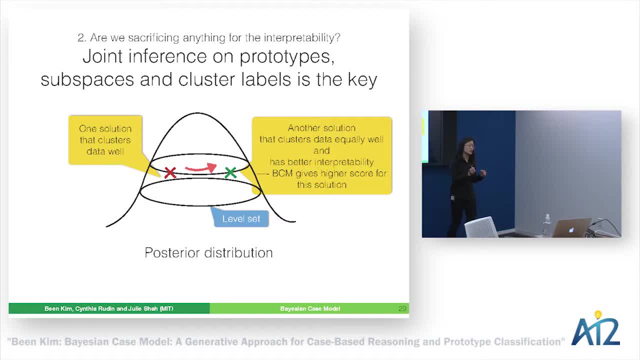 steps to do is to move, pushes, the solutions to a space where it is good- good clustering results, but at the same time, that clustering results can be well explained. and the key of doing that is the key is that this is only possible because we are 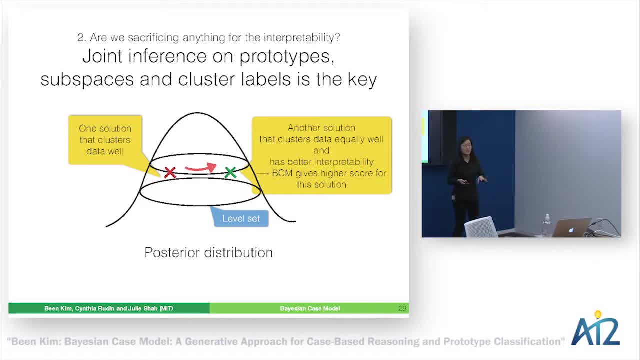 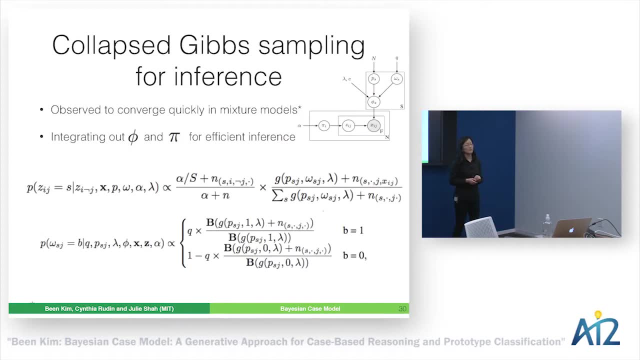 performing joint inference over the clustering and the explanations. If we are doing this as a post-processing or any other way of doing this, this may not happen. Yes, So it seems like you would imagine that there should be some way, like you said that it was. 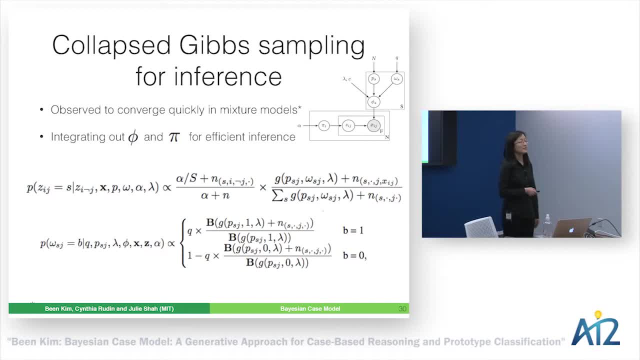 very robust to parameter choices, hyper parameter choices. It seems like there should be something in there that could tune your bias toward interpretability versus fitting the clustering, and that seems like that doesn't seem to be the case. Interesting, Yeah, so if? 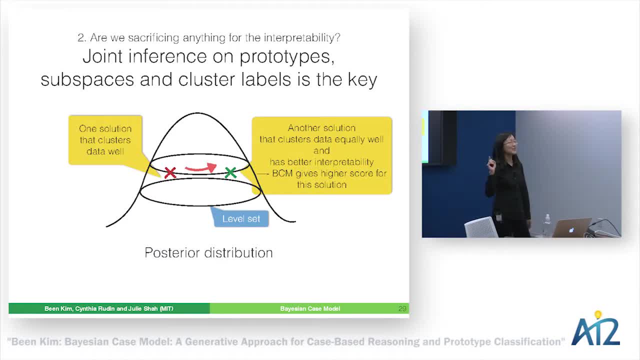 if this hypothesis, which we have not proven, is correct, then it's it's. it's not the case, right? So that that your comment is about. that assumes that there has to be some trade-off, but for this data. 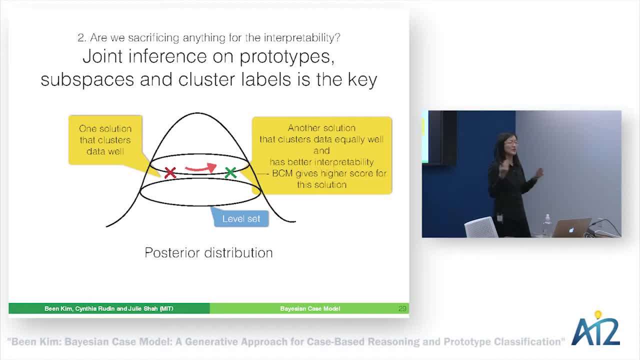 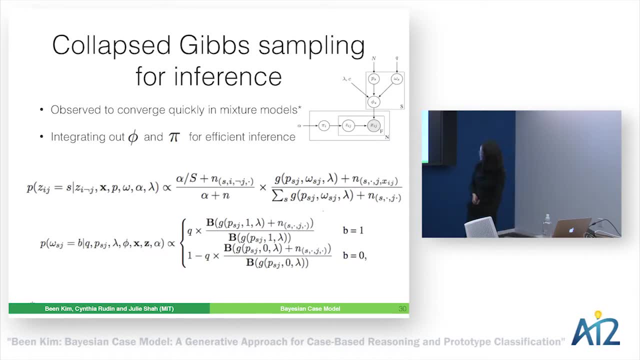 that we tested and for the settings that we tested, it seems like it just acts like a temporalizer. Okay, so these are. these are the collapsed Gibbs sampling. So we- we used collapsed Gibbs sampling for the inference. I did not mean to explain. 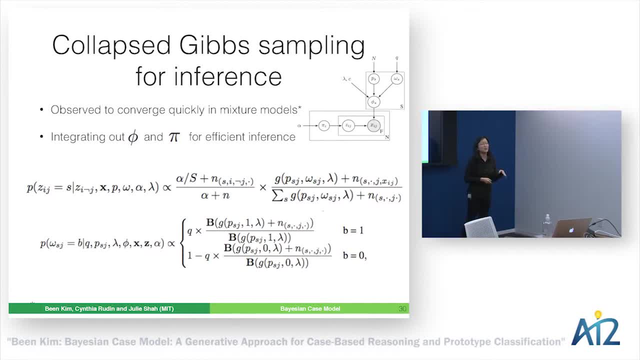 all this to you in in, in detail, but these are the equations that we used. We integrated out variables that we don't need- phi and pi- but you can always forward sample after you got other latent variables, if you are, if you. 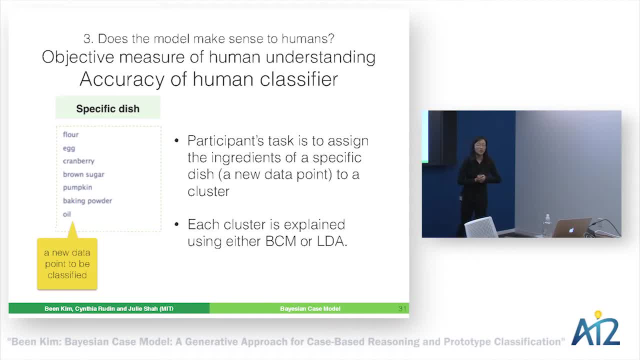 if you want to know about phi and pi, you can always put on your and and and, and and and. just, just, just, just, just a little detail. just a little detail that will be helpful for people that might like requires good understandings of clusters, And that's what we did. 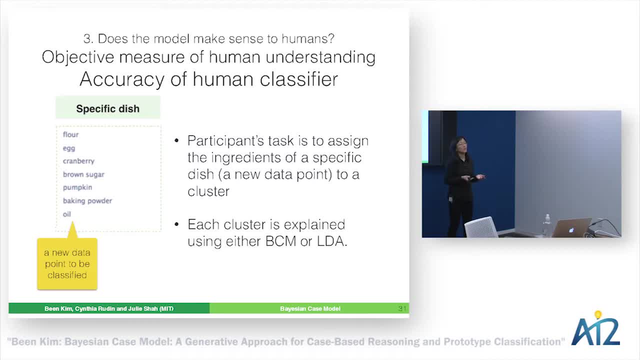 We asked humans to be a human classifier. We gave them a new data point, which is recipe data in this case, And we didn't show them the name of that dish, We didn't tell them it was microwave brownie, But we showed them the data points, the list of ingredients. 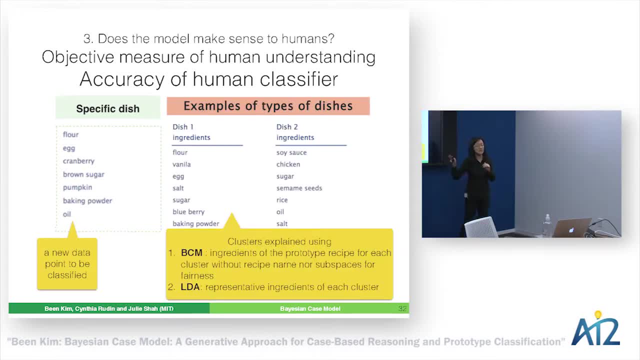 And then we explained each of the clusters using BCM and LDA. So half of the questions that subjects got were BCM And the half is LDA And the order is randomly chosen And we asked them to classify this new dish. Where does this new dish belong to? 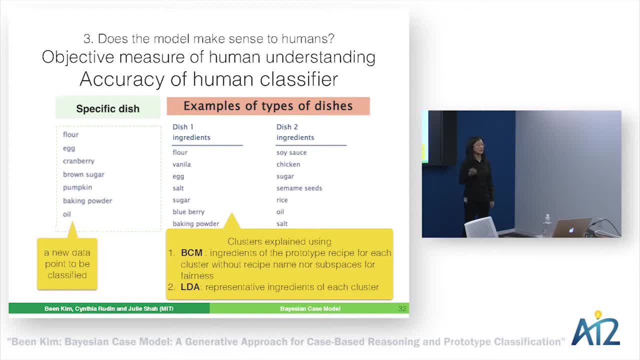 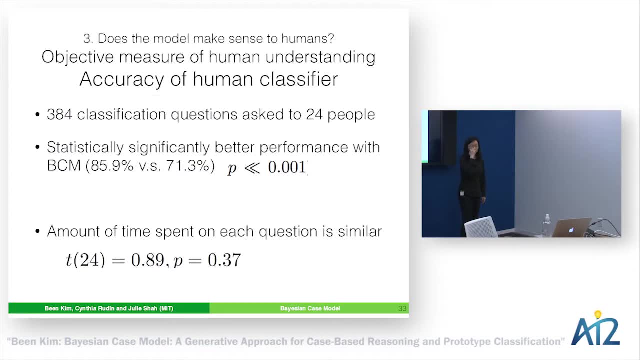 We showed four to six different clusters, all of which are explained using BCM or LDA. So we asked 384 classification questions to 24 people And the results we got was very promising. People perform statistically significantly better when they are using BCM. 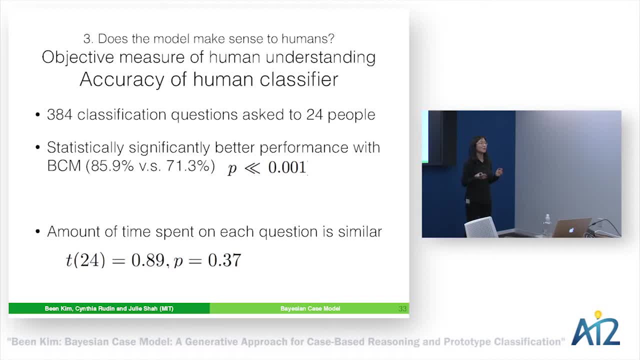 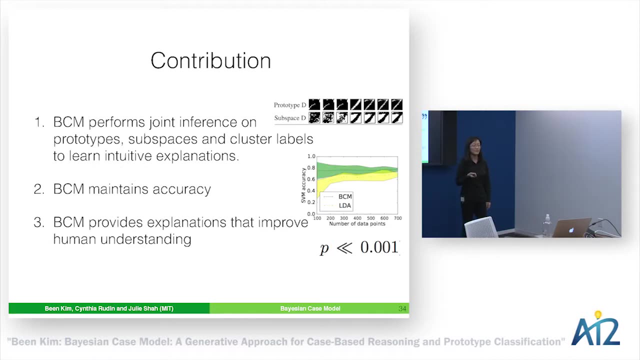 And they spend roughly the same time solving the problem. So this is preliminary results on: yes, the BCM explanations that is provided by BCM make sense And it can help humans understand things better. So today I talked about BCM And I talked about LDA. 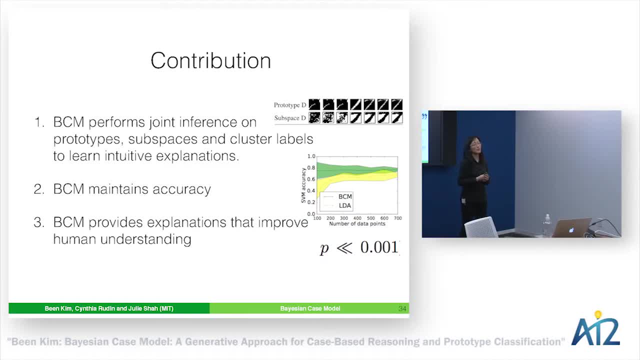 Part of my thesis work on making machine learning models that could provide explanations- intuitive explanations- to humans about the machine learning results. I showed that Bayesian case model BCM performs joint inference on the explanation and clustering. It maintains accuracy And it can provide intuitive explanations. 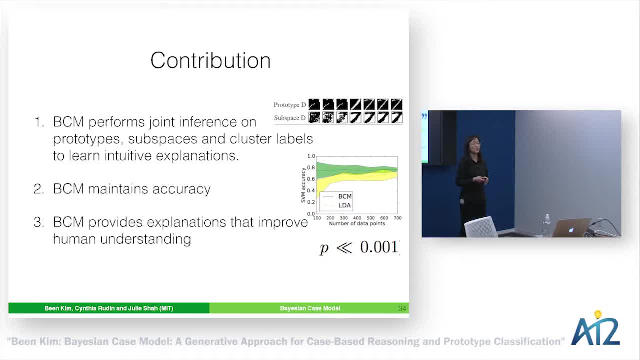 that could further improve human understandings about the machine learning results. Yes, So it seems there's a part of BCM coming from the fact that, because you require these prototypes to be actual examples, when you do your sampling you're jumping across spaces, unlike in mixture models where you have incremental changes. 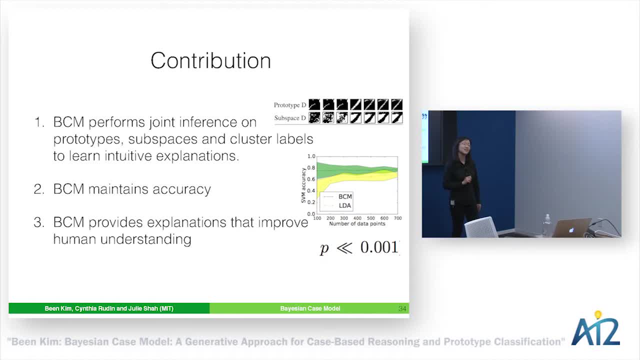 Yes, And this leads to the question: do you think there is an issue when you have fewer examples? It doesn't appear to be the case in your graph, But when you have fewer prototype examples, do you think that would cause an issue with BCM? 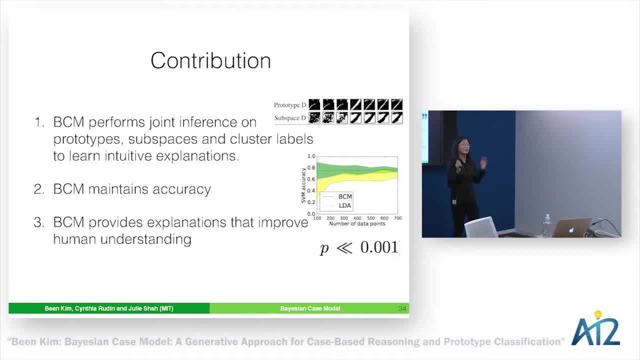 Oh, like fewer clusters, Like you said, that You said to BCM. we only want to learn two clusters, for example. Or you have only three examples for a cluster. such like the mean of the three points might be a good representative of what 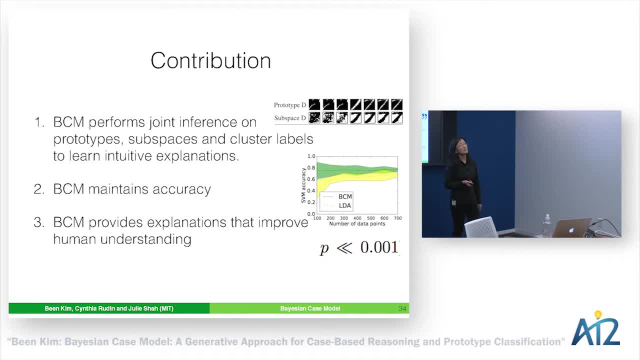 a mixture model would find, But with BCM you have to pick one of these three. Oh, I see. Yeah, that's a good question. So I think there are two questions in this. The first question was: is it using? 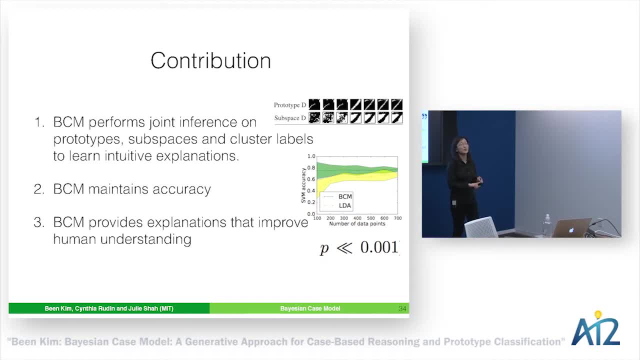 sort of leveraging the power of the fact that you have to pick the real examples? And second is what happens if there are not that many data points belong to a particular cluster? So to answer your first question, yes, I think that's what might be happening. 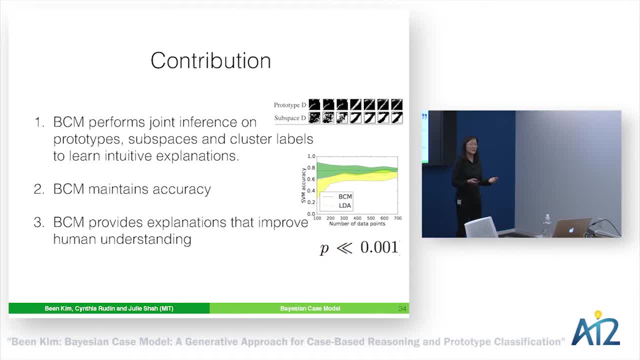 What LDA or other models that uses a mixture model. what happens there is that you completely ignore, for the computational reasons and reasonable assumptions, oftentimes for real data too. you assume all the features are independent, And we do that too here. 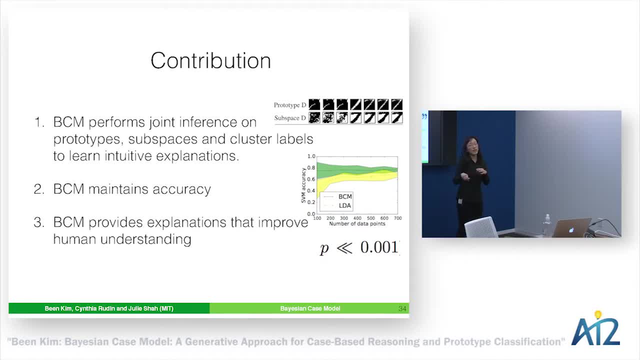 But indirectly we kind of capture relations between features because we have to pick a data point. So if there is a data point, there's no data point, that feature one and three happens at the same time, then that's going to get a less score because just simply there. 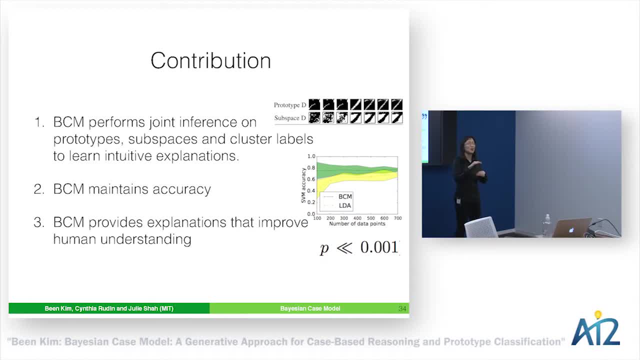 is no data point. So we kind of capture the relation between the features or maybe correlation between features, because we are modeling, characterizing clusters, using examples. For your second question, because there are three questions, so I think that depends. So let's say you have three data points in one cluster, very, 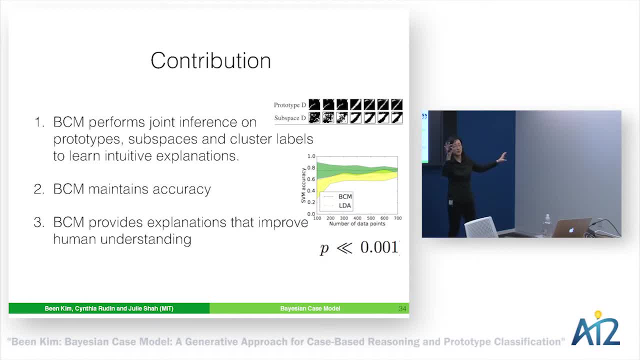 far away and all the other guys are pretty well-defined here. five clusters, 100 data points each. right, I think it depends on how close these guys' three data points are for the rest of the guys. Again, I think it's similar to the challenges. 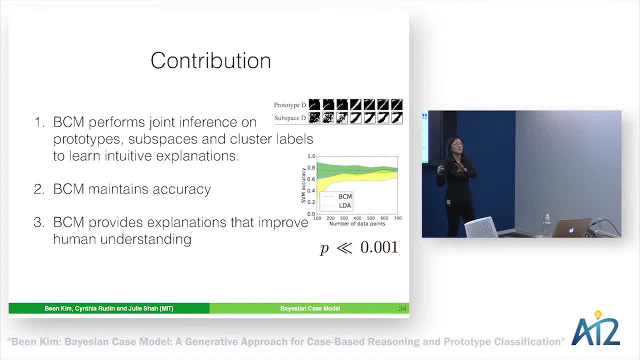 in regular clustering algorithms where if it's close it's just going to be observed by these rest of the people. If it's really really far and it really scores very poorly on the other clusters, when we are doing kip sampling, then it's. 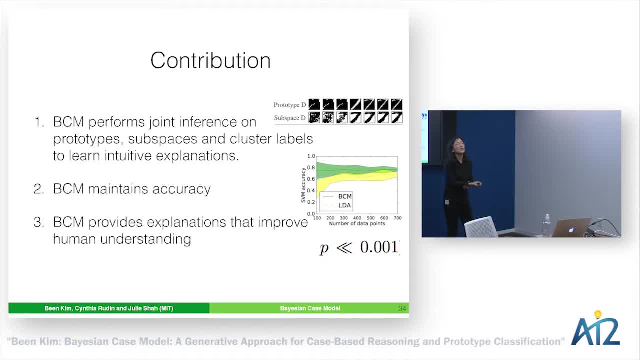 going to try to form a new cluster. I don't think that because we are using prototypes, it might benefit a little because there is an actual example that could well describe that cluster, But I think same challenge of identifying that cluster is going to be there. 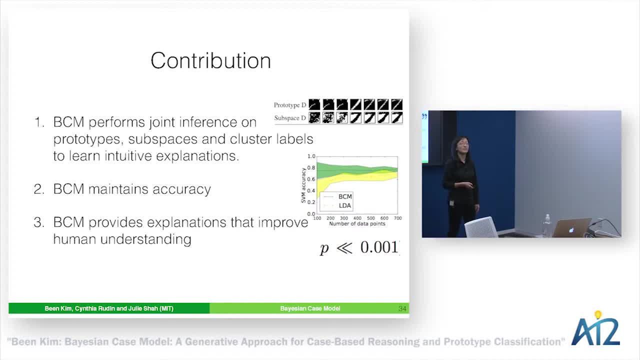 Yeah, My point was more about the fact that, because you're required to pick one of these points, the mean of these points would be a better representation than picking any one of these three. Why do you think so? Spread out, Oh, OK. 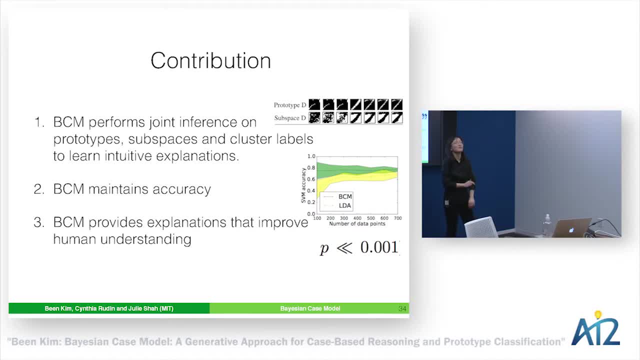 Like, if there is this picking, this might be better. If you had a lot of points, then you could potentially get that centroid as your prototype and you're happy. But if you didn't get the centroid in your prototypes then you would start with picking NXP. 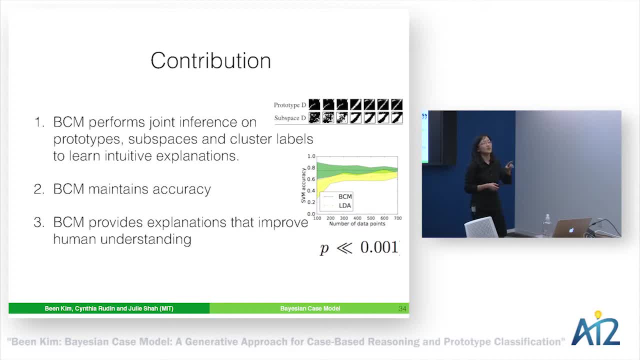 That's right. That's true. That's true, But I think I can argue that that is true. I think it might be poor representation if you calculate the distribution over this and the score absolute likelihood might be lower in the case of picking the prototypes. 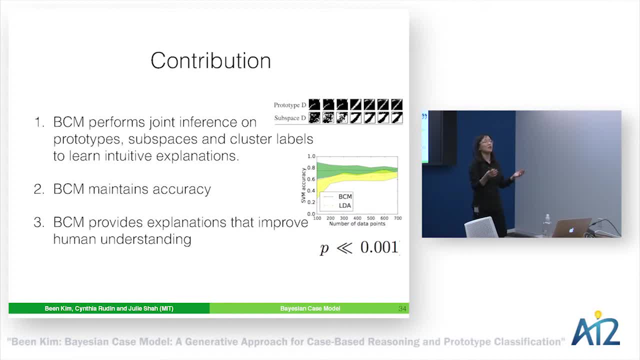 But in the scheme of the things, if that really makes that much difference- picking one data point versus picking the middle of the data points- then you have three data points that are really far away from each other, So maybe they shouldn't be in the same cluster to begin with. 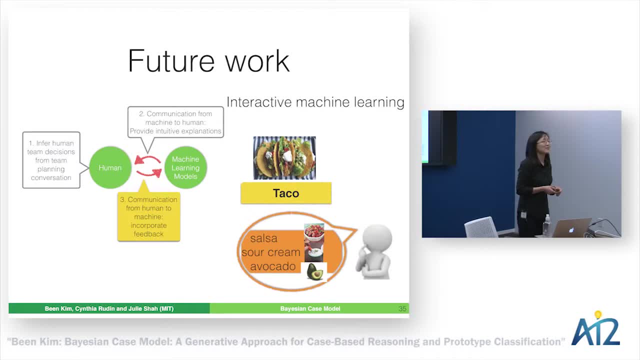 OK, So future, yes. One more question. So a lot of the LDA work in sort of recent years has been more on optimizing hyperparameters. Like, if you take the number of clusters properly, the cluster is actually not being better than if you had the wrong number of clusters. 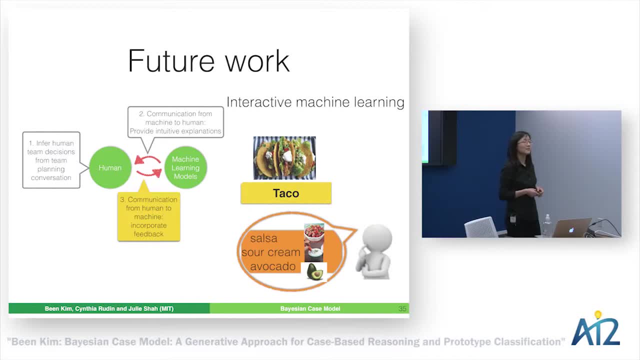 Right, right, right. So the evaluations you have right now is: you pick the same N and you compare it against your LDA. Have you tried to put that within a hyperparameter setting where you try to optimize big N and does BCM still? 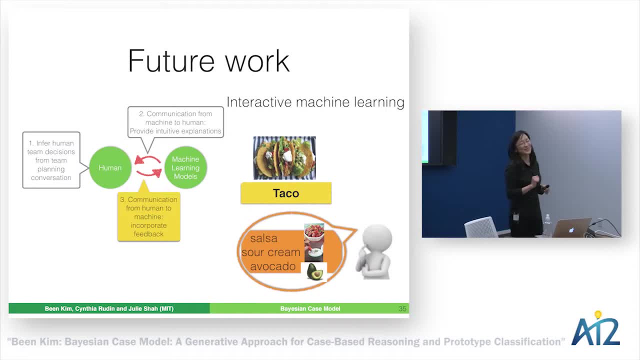 perform better. That's a really good question. I'm glad you asked the question, So I have not Answer is that? But all the really lots of literatures on LDA picking, non-parametric business, all the Chinese restaurant processes, Gaussian processes for optimizing hyperparameters? 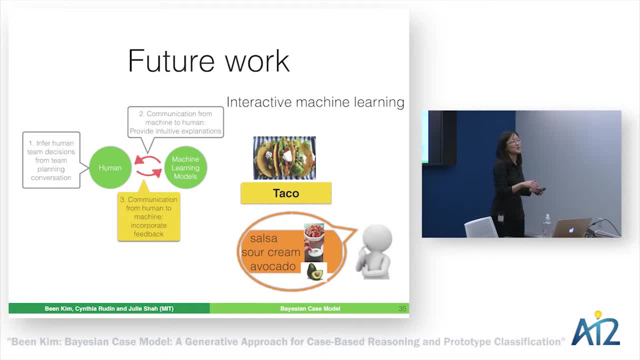 by work by Ryan Adams at Harvard. all of those are applicable to BCM. So picking the right number Of the hyperparameters. those techniques are really well studied, widely studied. We can leverage that. But how well does your algorithm? sort of plus the right word be great if you pick the wrong N. 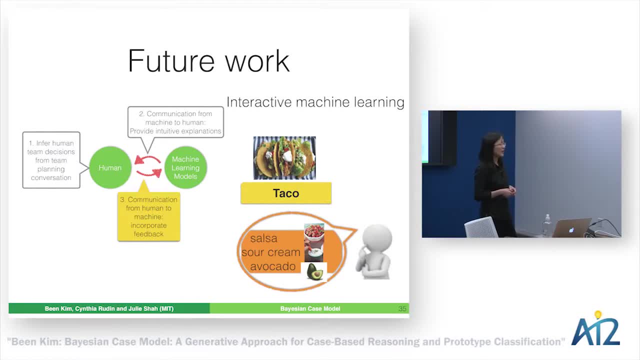 So I guess that's the question. I see, I see That's a good question. I don't have a plot here, but I did plot number of clusters with the likelihood whether it does it. is there a switch zone that we can pick? 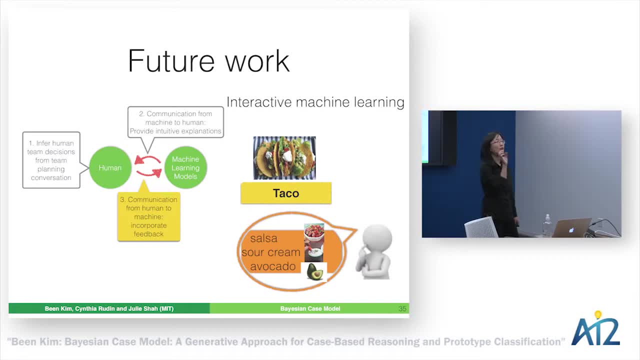 whether avoiding overfitting and underfitting, right, But there. So there exists that cluster that we see. pretty much the same pattern as LDA is what I was trying to say. So we'll see. if you pick too many clusters, it will overfit. 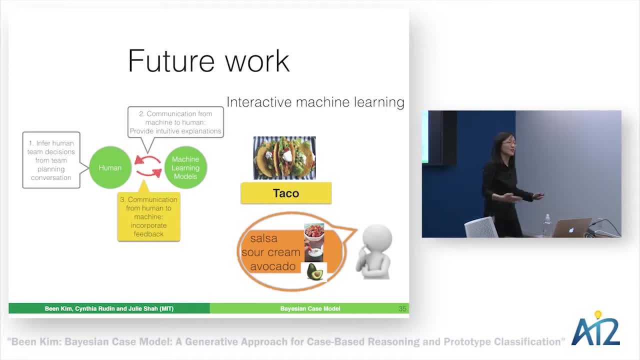 It behaves a similar way because the way that we model the underlying data distribution is exactly a mixture model. So I don't expect it to be- I haven't tested, but I don't expect to be- dramatically different than other generative models that leverages mixture models.